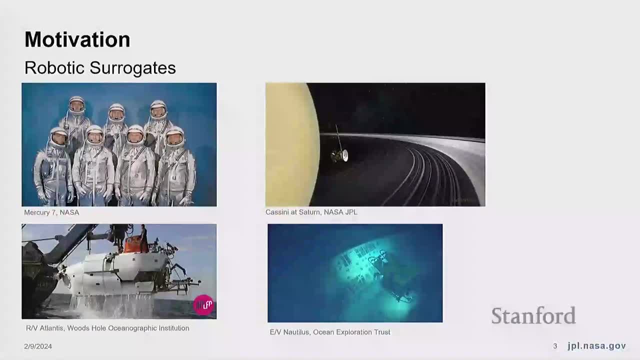 with the Mercury 7 and the Alvin, which is a deep sea human-operated submersible. But, as you know, some of the challenges that we're going to be dealing with today are going to be very, very extreme, And the challenges in these extreme environments include pressure. 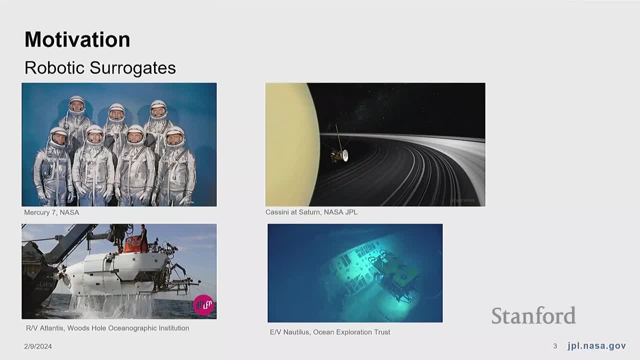 temperature and radiation, often to very extreme levels. There's an anecdote that at some point during sending robots into Fukushima after the incident there, the hardest part of that challenge was actually avoiding all the basically failed robots on the way in. just due to the extreme radiation environment would fry a lot of the computers and components. 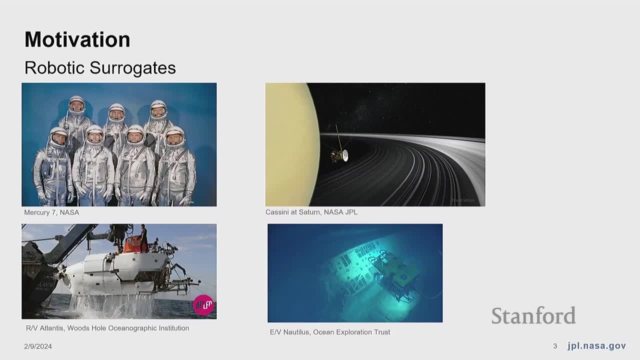 So in the lab we're spoiled. We have the best computers, the best sensors- They're plugged into a wall. We have nice environmental controls over the lab. So we get to do all these advanced and great things In reality, in the real world, as you put things further and further out. 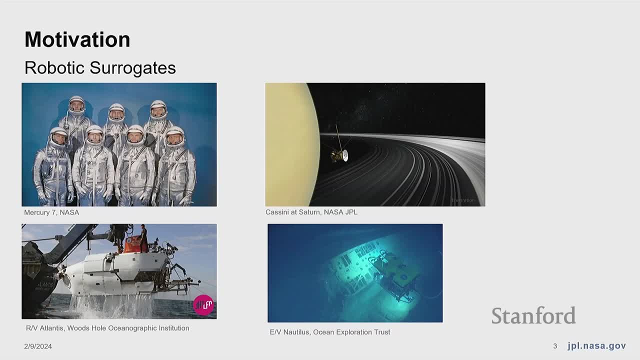 into the field. every sensor, every actuator, every computer comes at a cost to the mission. That can be in terms of dollars, It can be in terms of mass, It can even be in terms of science return. If you have to heat an element versus use that same limited power. 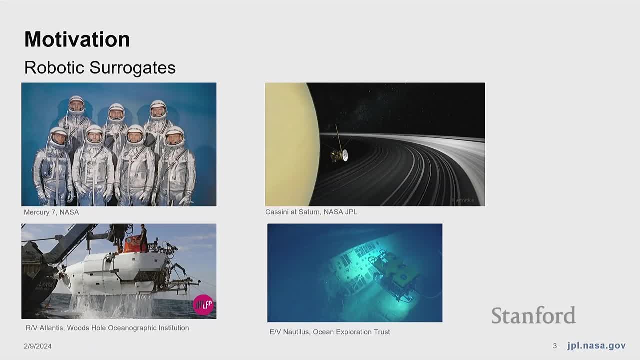 to run your primary instrument, you potentially have direct damage to the instrument. So that's the main challenge, And then the second challenge is the cost there. So all of this puts a premium on simplicity. It motivates. how can we look at pre-programmed structures? baking intelligence into a mechanical 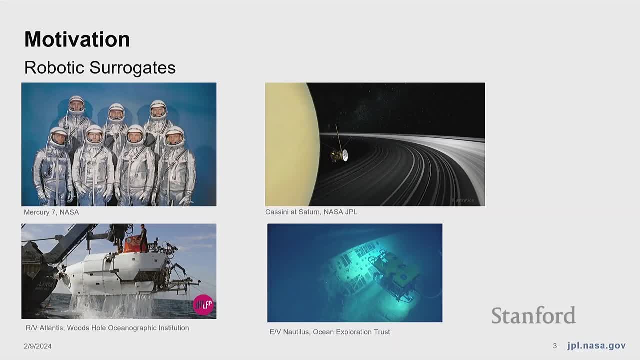 design itself to eliminate some of the need for fancy controls and all the best robotics that we often see in more benign environments. How can we actually reduce the requirements on, especially along the extremities of a robot itself? So I'm going to go over a few projects from my PhD research, with an emphasis on soft. 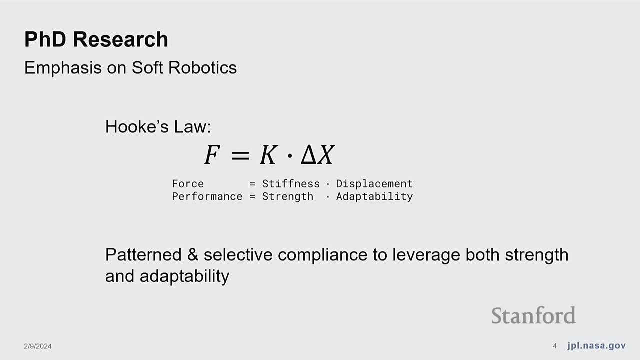 robotics. You're all probably familiar with Hooke's law, which is basically that the force is going to be proportional to the stiffness and displacement. So for a fixed force, there's this direct trade-off between your stiffness and displacement And I see this as a useful 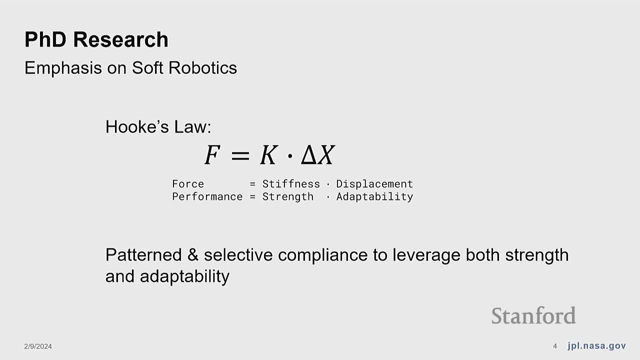 though somewhat simplistic approximation for the field of soft robotics itself. But there's typically this trade-off between strength and adaptability. So the stiffer a robot, the higher loads it can support without deflecting, but therefore you have less room to actually comply and adapt with the environment itself, And then the performance is analogous to being 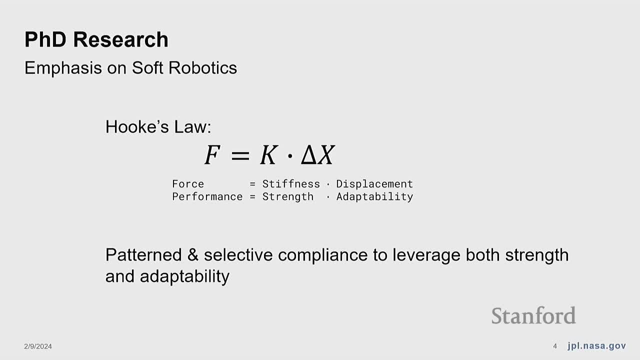 the combination of those two. So again, if you treat your stiffness as a linear approach, you're going to have a fundamental trade-off here between strength and adaptability. But if you look more at how can we pattern and selectively choose where our compliance is, how can we then leverage both strength? 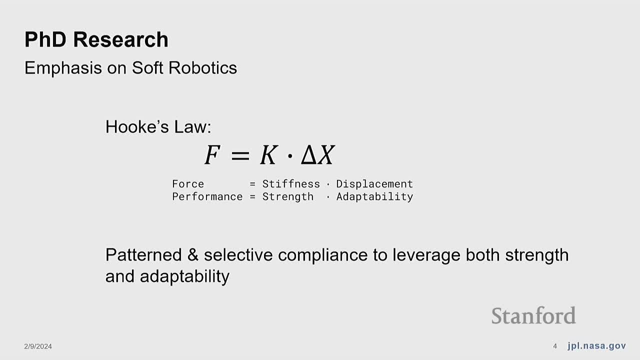 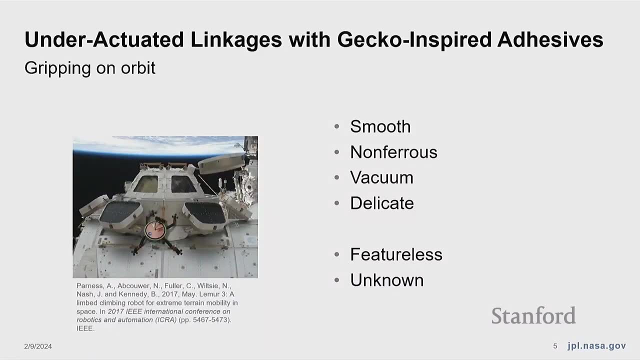 and displacement. And then the third challenge is: how can we look at, how can we pattern and selectively choose where our compliance is? How can we then leverage both strength and adaptability to get both parameters and increase our overall performance in these extreme environments? The first project here, put very simply, is: how do you grip things in space? This is a 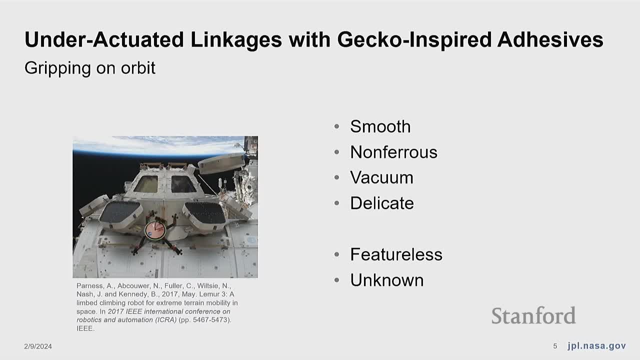 fun challenge, and fun being another word for difficult. There's plenty of complicating features here. A lot of spacecraft are smooth, non-ferrous. You can't use magnetic approaches. You're in a vacuum, so you can't use any kind of suction. 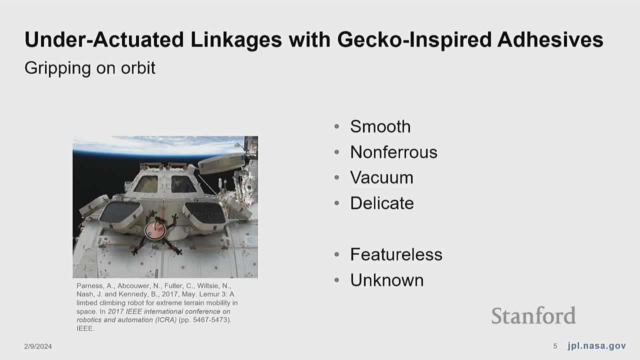 As well as having to avoid and be concerned about delicate surfaces. Additional challenges include the fact that a lot of objects and areas of interest for gripping are featureless and potentially some of the best applications in on-orbit gripping you potentially are dealing with unknown shapes and objects. Again, some of the best applications here are satellite. 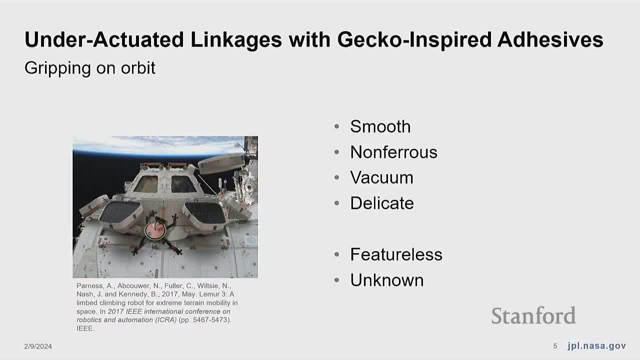 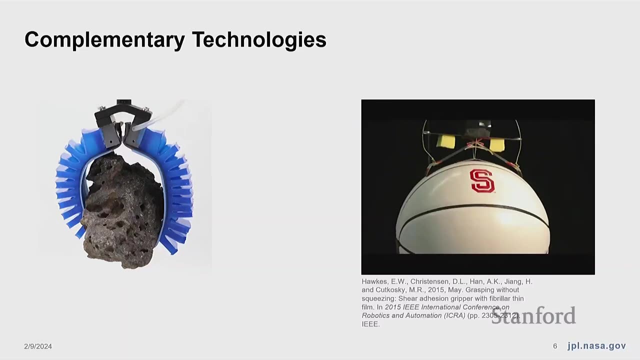 service and repair, in-space inspection and maintenance and then de-orbiting space junk, and in all those use cases you potentially don't know exactly what your target operations are going to be in advance. To look at this problem, we were motivated to look at basically two complementary technologies. 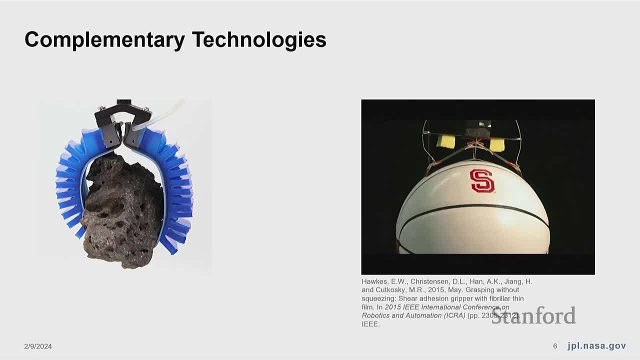 looking at both elastomeric, flutic elastomeric actuators and then gecko-inspired adhesives. They both offer some similar advantages and then unique challenges and specialization as well. So the soft robotic actuators. The soft robotic actuators offer compliance at a fairly large size scale. They have innate. 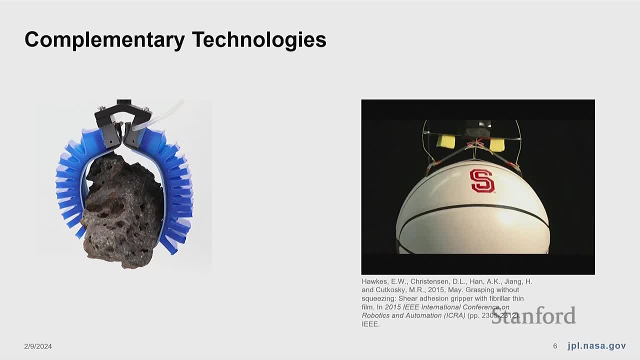 ability to be simply controlled, yet adapt to the shape of the object that they're gripping, And similarly, a lot of the fantastic gecko-adhesive research here has actually similar properties, but at a different size scale: The ability to adapt to microscopic roughness and, through that process, exploit van der Waal. 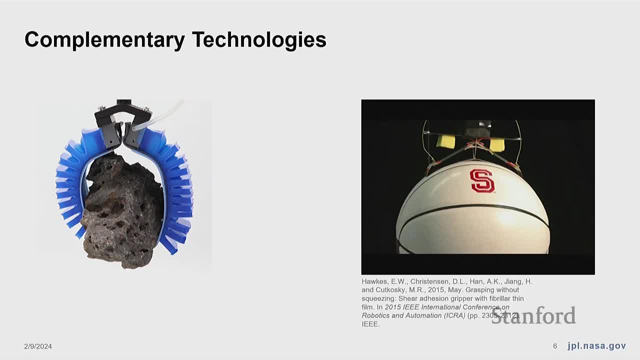 forces And wrap and engage and support high loads, But then they do offer each challenge as well. So gripping on again. for the soft robotics, any kind of strength does present a challenge because you have that lack of stiffness. And then for the gecko-inspired adhesives, really again, they work through this van. 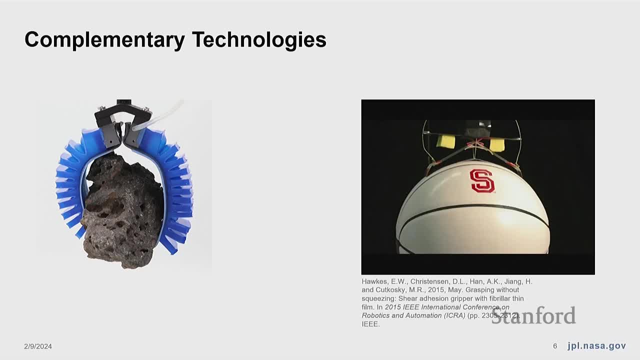 der Waal forces, which are weak intermolecular bonds, And so to get those you have to rely on very close surface contact. So we looked at how you put these together And basically promote the structure, Promote surface contact on an unknown object. 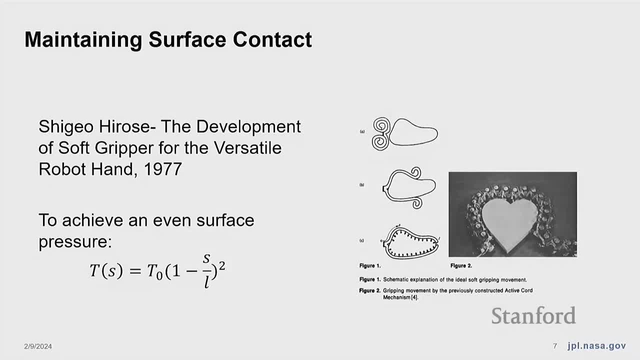 Luckily, to answer this question, we had a great pathway forward. Shigeo Hiroshi researched this topic back even in 1977, looking at how do you maintain or achieve an even surface pressure distribution across an arbitrary object with a continuum, And basically making several assumptions. and we're gonna come back and look a little. 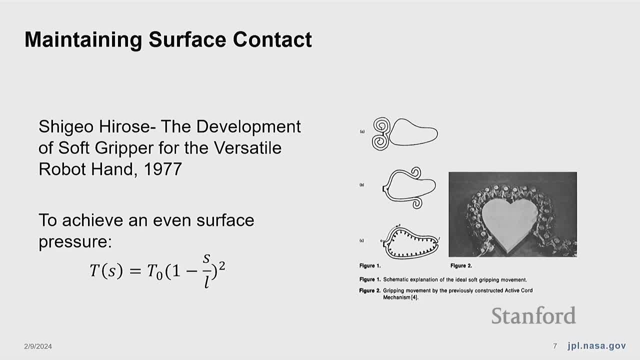 bit more at these assumptions later on, But for now we can just treat this as a good starting point. To achieve this goal, you basically need to have a beam or actuator with a torque distribution as described in this profile through this equation on the bottom left. 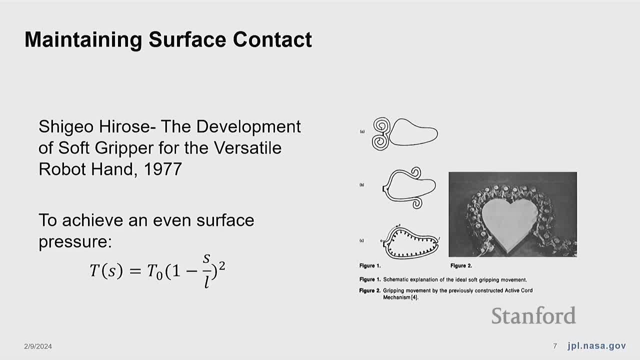 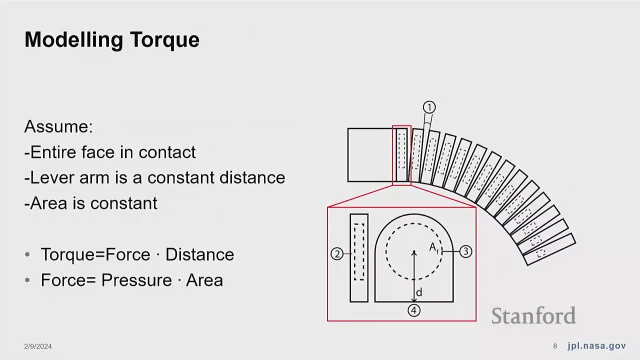 Basically, this just means that your torque is going to be exponentially decreasing from the base to the tip of the digit. So, looking at how to apply this to the field of soft robotics, there were a lot of great models and there still is a lot of great model development. 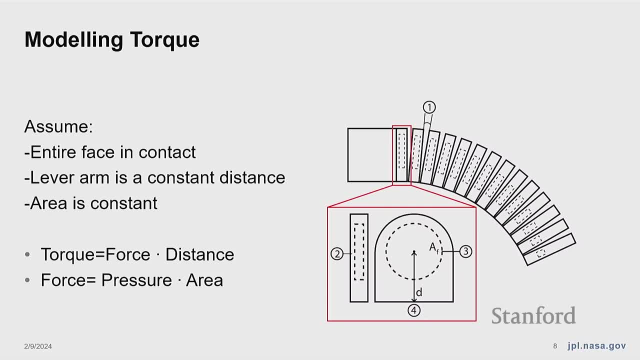 But most of the models were: if you take a design, then you can do work simulating and predicting what it will do. We wanted to go in the other direction: have a model simple enough that we could use it during our design phase to actually get the behavior. 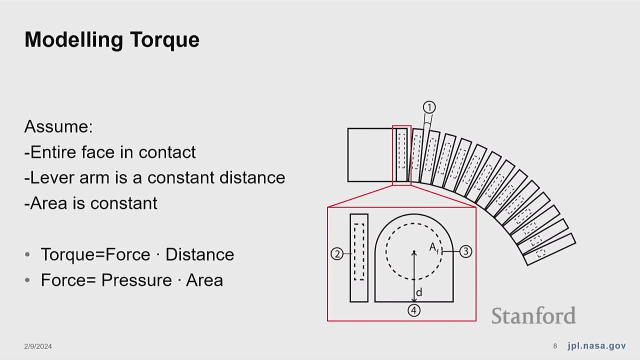 that we were after, which, again, is that even prescribed torque distribution? So we treated this basically. we looked at how can we make a model simple enough that we can use it in our design phase, And to do that we basically idealize a fluidic glass. 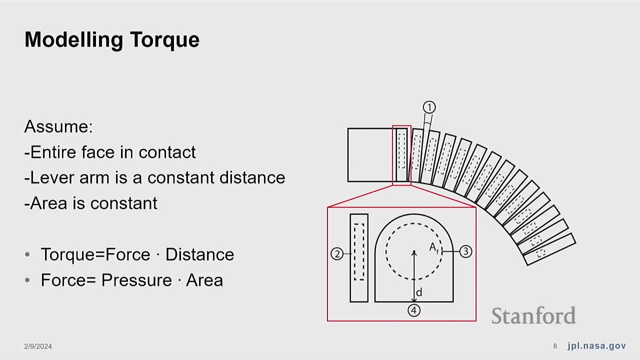 and actuator and assume that all of the torque is coming from these individual, discrete joints that are occurring where the faces of two adjacent joints are pushing together And at that point you basically can treat it as a pretty simple problem. where the torque is going to be, the force times the distance of the moment arm. 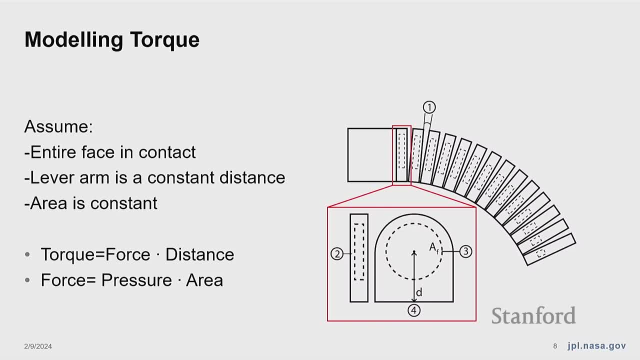 and then the force is going to be the pressure times the area. So, really looking at simple math, to solve a complex behavior, To try to adhere to this model we actually have to make and then design our robot to try to maximize these assumptions, which 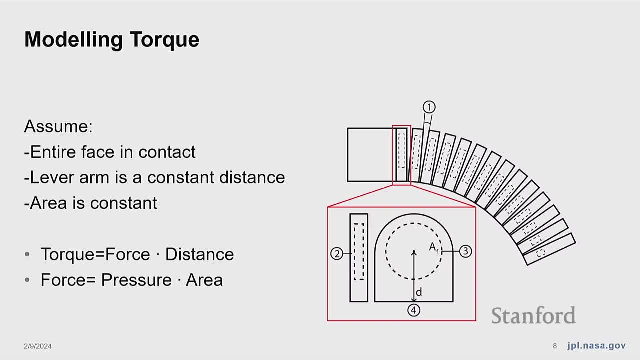 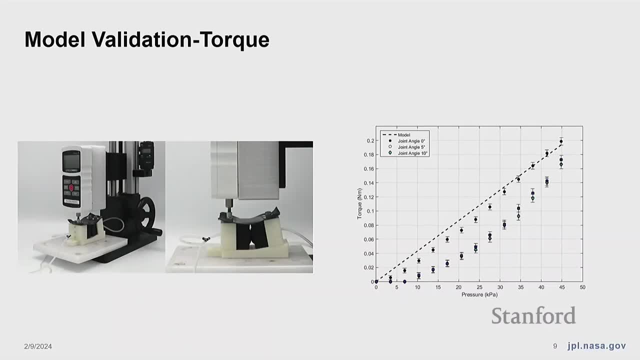 is assuming that the face is in contact, that the lever arm is a constant distance, that the area is constant. As you'll see in this slide, there's of course problems with this modeling approach. It's far from perfect. There's two main dependencies to cover. 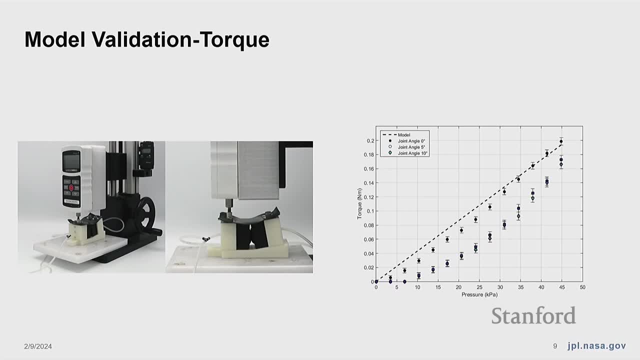 First is that there's a strong angle dependency, So, as you have joints that are separated by some angle, it takes further pressure and basically stretching of those faces to come into contact. And then the second is just the pressure itself, So as these faces are expanding, both their moment, arm and area. 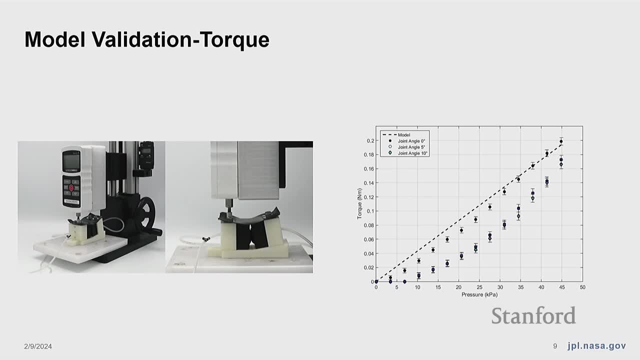 and contact are changing as well. So there's two main dependencies here- angle and pressure- And you can see their impact. But we thought generally this is not too far off, And let's look at what this looks like over the entire gripper. 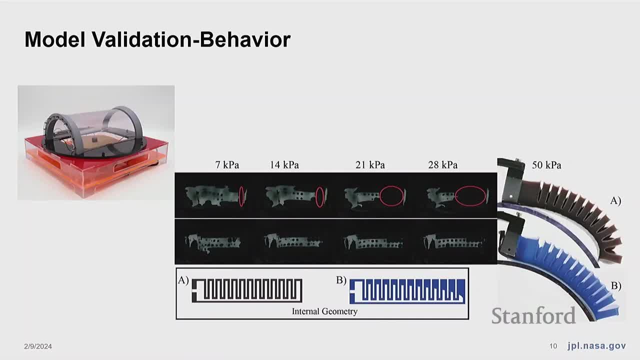 So, again, the behavior that we're after is maintaining contact, And what you see here in this slide are two different grippers, with the only real difference being the internal structure. On the top in part A, you see a gripper that has a uniformly distributed internal geometry. 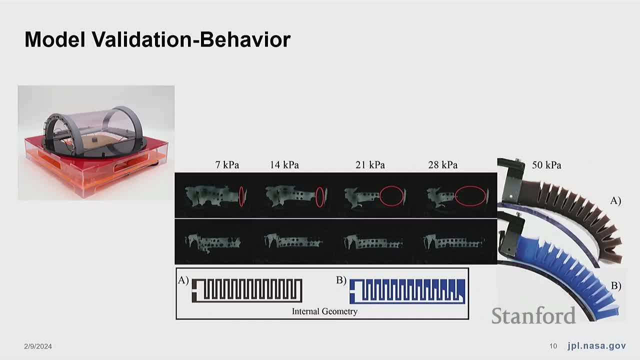 So each chamber is the same size as the next And in the bottom you see the gripper that has been designed to this torque profile using the model, And what you see is basically what you would predict: that as you inflate and increase the overall torque in the gripper on the top, 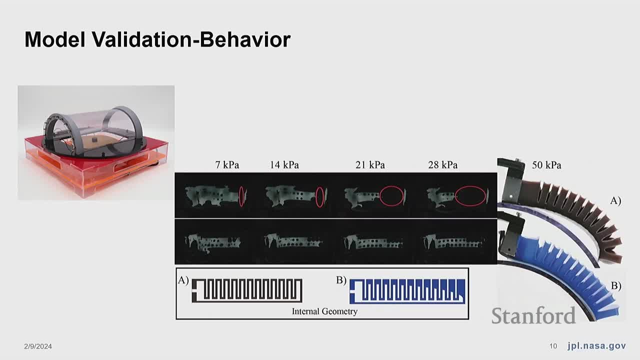 the distal joints have enough torque because they all effectively have the same torque. It has enough torque that it can then force off the rest of the finger And you lose that contact that's required for engaging the adhesives In the bottom. you see that you're actually able to maintain. 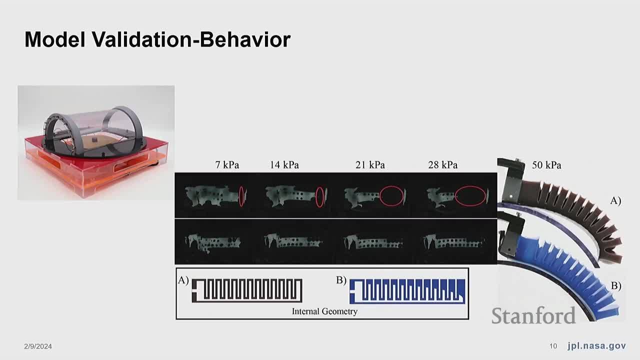 this even as you increase the torque across the gripper. We validate this through looking at the real surface contact area, which is done through a custom-built cylindrical, frustrated total internal reflectance sensor. So basically, we have this edge-lit polycarbonate tube. 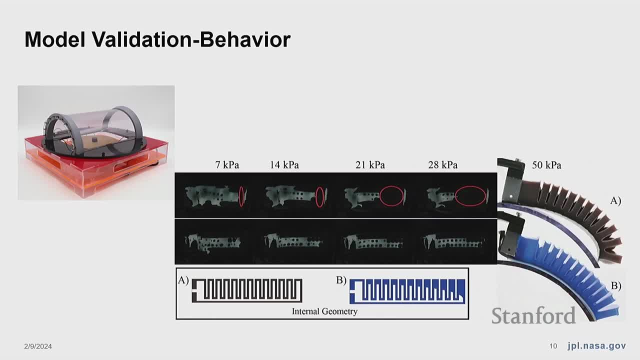 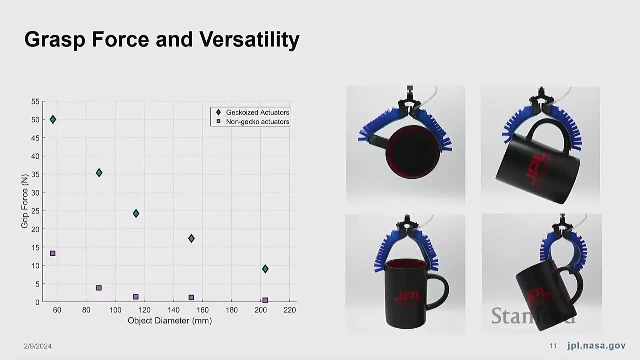 in a dark room And, using that, the only light that escapes is what's actually in contact with that surface. Then we looked at the behavior and performance of the gripper with the gecko-inspired adhesives. as a whole, You see a few interesting things at all size scales. 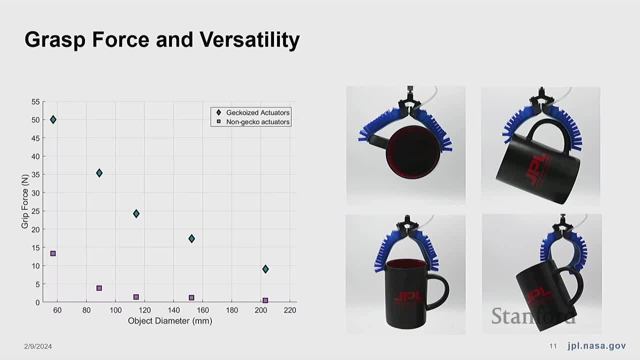 The gripper performed better than the similar one without the gecko-inspired adhesives. The other thing, you see, is a large dependence on the size of the object that you're gripping. So these adhesives have a very interesting property. Often we think of friction as being something 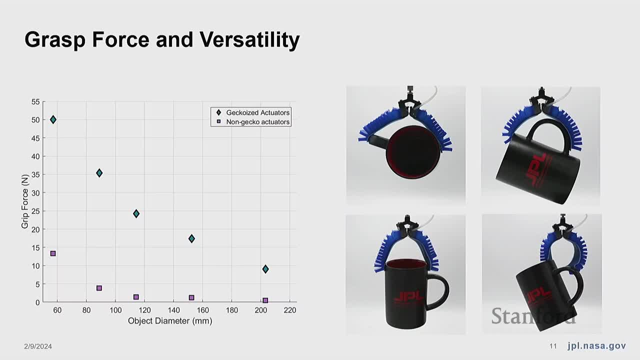 that's load-controlled, So the harder you squeeze it, the more frictional force you get. Some of the magic of these adhesives is that they actually have adhesion-controlled friction, So you don't have to squeeze an object to be able to get. 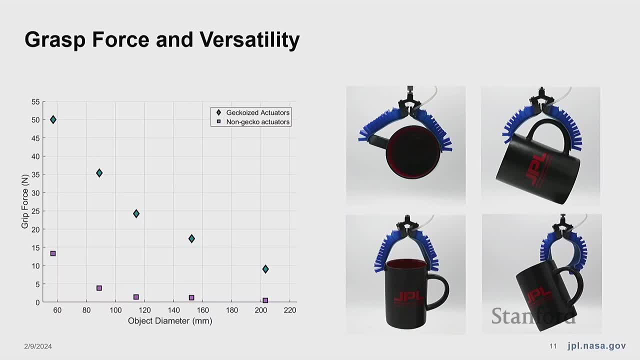 this high adhesive force, And an interesting and great way to exploit this is by wrapping around an object, You're creating these frictional forces tangential to that object at all points along contact. So what this means is, if you're trying to grasp a cylinder, 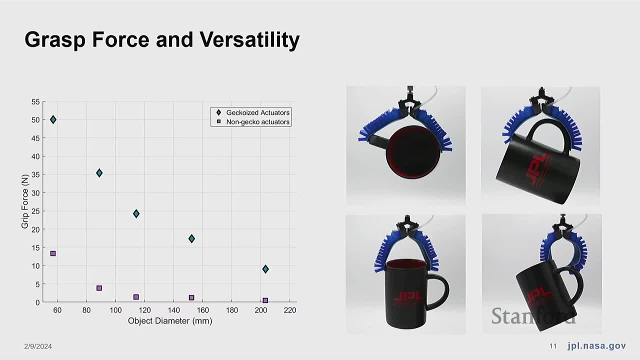 near the middle point of the cylinder you have more forces that are pointing upwards that can actually support vertical load. But as you get closer and closer to the top of that cylinder those forces are really pointing horizontally and you don't get much strength contribution from that. 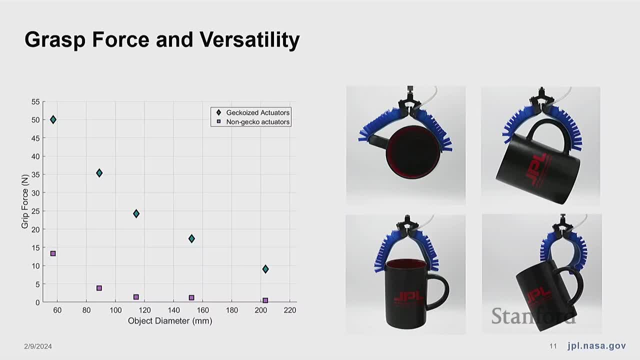 So there's this inherent size dependence. when you're gripping something in this way, The other thing you see on the right is we wanted to look at overall grasp options, performance and versatility. So what does this kind of gripper enable? And we see that it enables grasps. 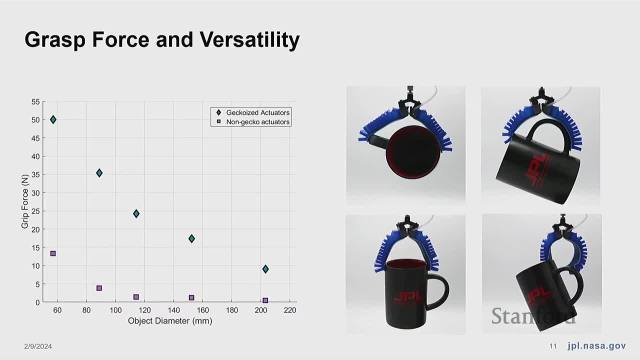 that you couldn't do with either technology before. So there are a lot of cases that we found that you have a hybrid grasp where one finger is providing a normal force or enclosure support and then the other finger is doing this surface adhesion and providing strength that way. 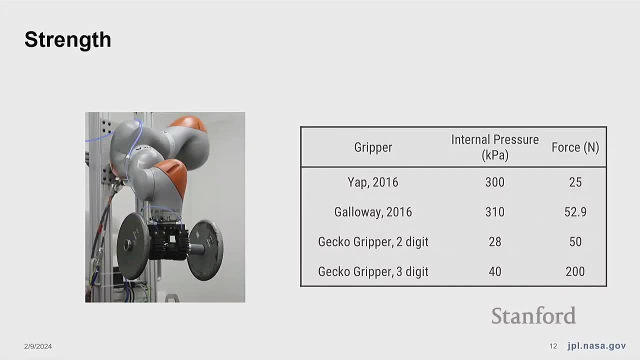 The next thing we did was we took our robot to the gym and saw how much it could lift. We had both a two and three finger version that we tested the maximum force on And a few interesting points here. So first you'll see comparisons. 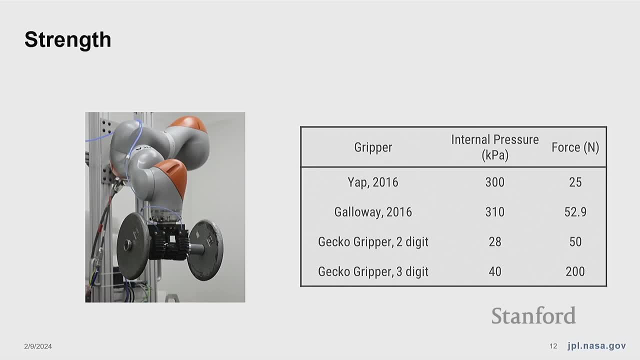 to some of the other state-of-the-art grippers at the time, And you'll see that the forces and loads that we support are similar, if not higher. And again, we were able to do this at low pressure, And that low pressure is key because it. 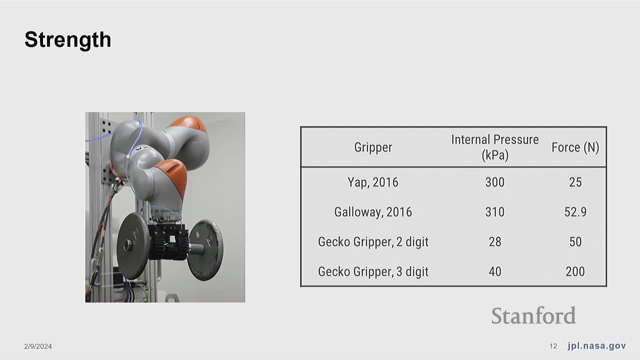 gives us two options right. First is it maintains the flexibility of the grippers, that adaptation, which is the whole reason that we're pursuing this type of technology. And then the second is that it's scalable. So if you want to increase your strength, 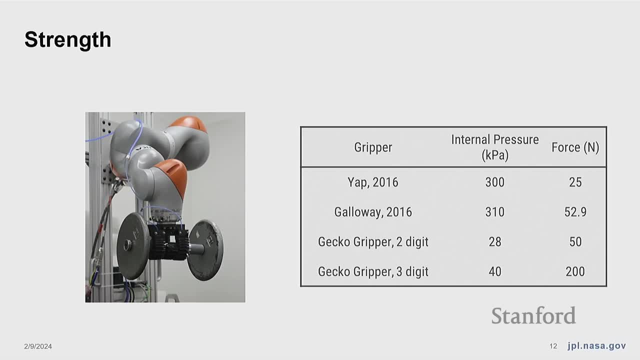 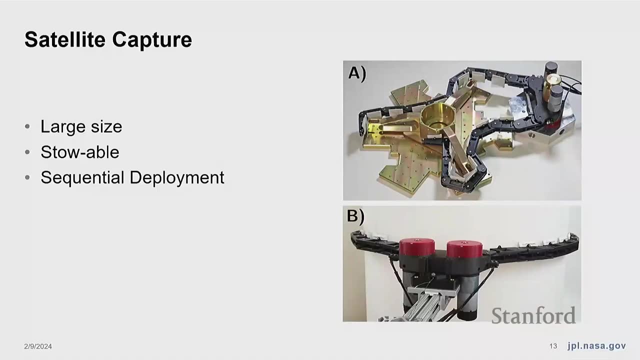 of the overall gripper. you need to scale your adhesive area, not necessarily the pressure and stiffness that you're putting into it. The next project that we looked at is: how do we scale this up in terms of size? At this point, we were interested in gripping. 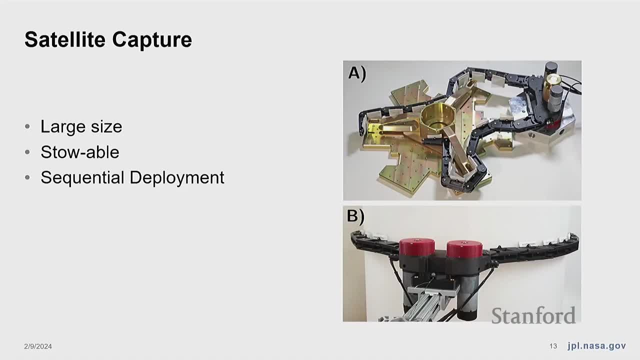 entire satellites again for potential capture and refueling. You can imagine it's much cheaper to potentially refill a propellant tank than send up an entire new satellite. So that's what we're looking at right now, And again we're looking at the size of the spacecraft. 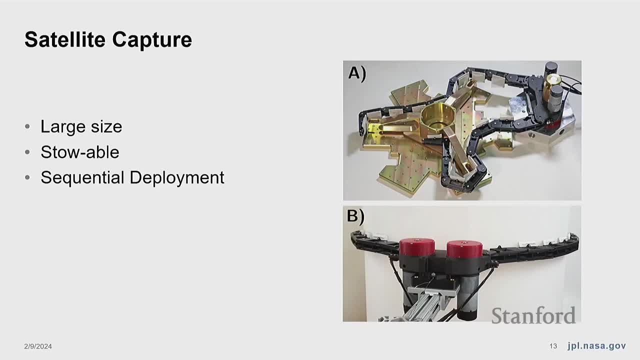 But capturing a satellite at this scale potentially motivates again a larger size, And this had a few new design drivers that we wanted to look at as well. So having something that was stowable and had sequential deployment again, and the sequential deployment was 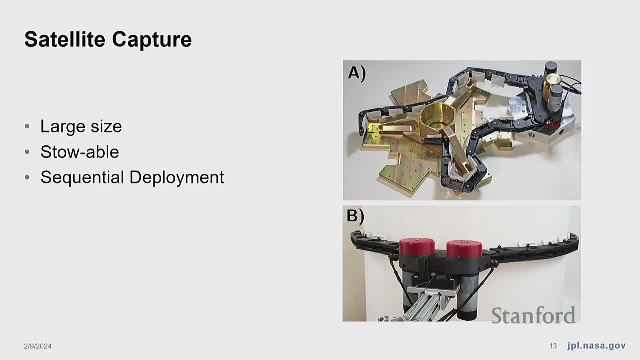 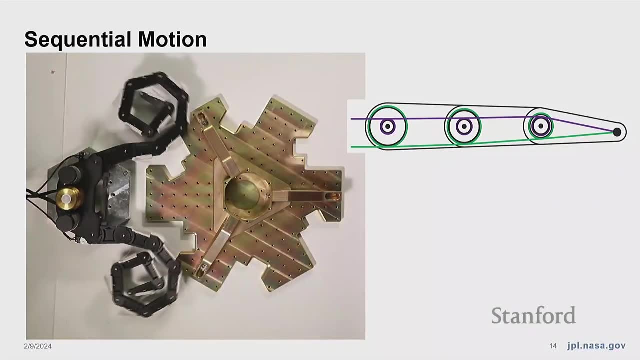 towards being able to conform closely to an unknown surface. So first I'm going to cover how we did the sequential deployment. So here you're going to see the gripper forming to an arbitrary object. This was a spare mirror mount that we 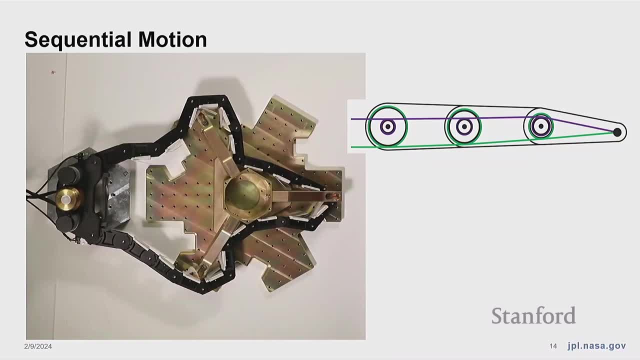 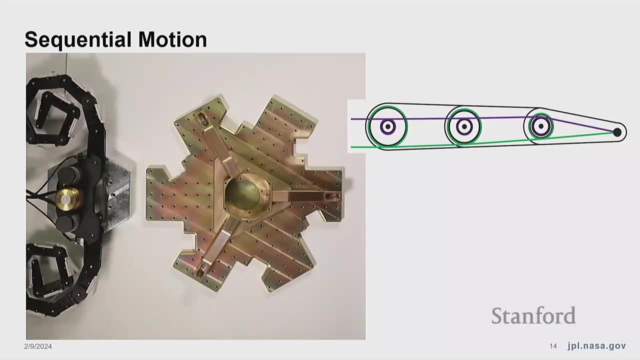 found lying around a lab. And the way that we do this, you see it retracts the same, basically the reverse process. So this is a highly underactuated gripper. It looks quite different from the pneumatically actuated version you just saw in the previous set of slides. 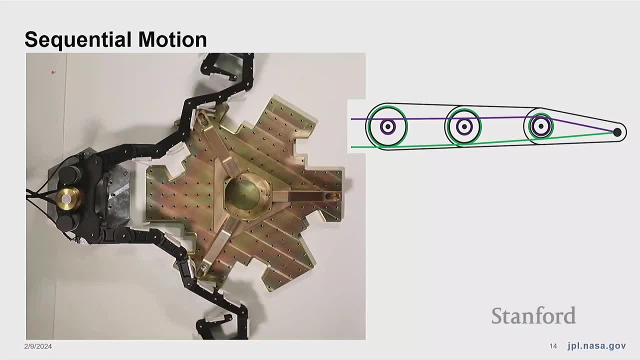 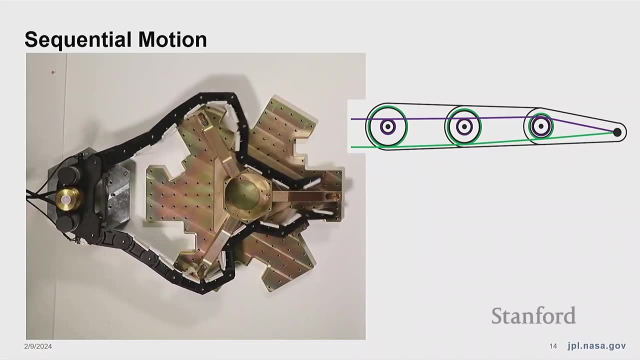 But there's actually only one actuator per linkage. So we have a single grip tendon running through this linkage, connected to a series of ligaments. There's a series of pulleys And then we have a passive retract tendon attached to a constant force spring operating. basically. 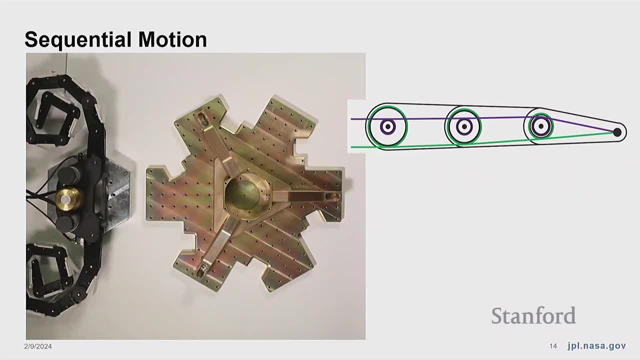 this retract And you can see basically the simplified version on the right. here is what these pulleys look like. So you have this retract spring providing a constant force and then uniform torque, with all the pulleys the same size, trying to torque each joint backwards. 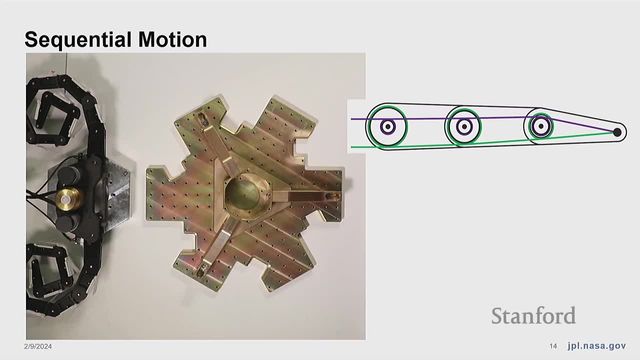 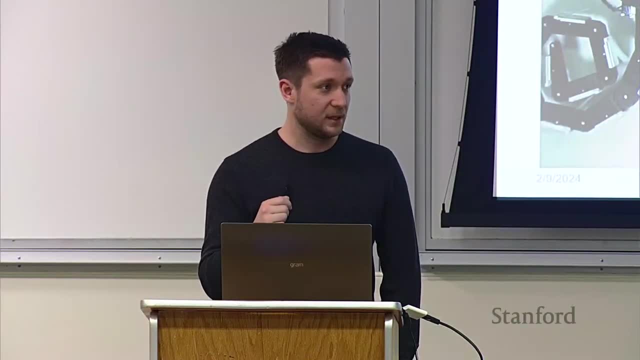 into the stowed configuration, And then you have a monotonically decreasing, say spring, And then you have the size pulleys on this grip side, And so, as you provide more and more tension to this grip line, each link, one at a time, switches over. 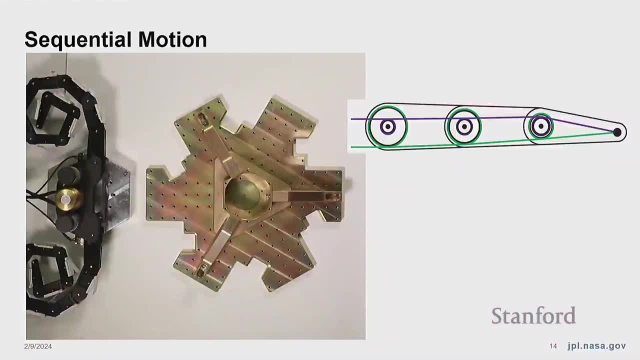 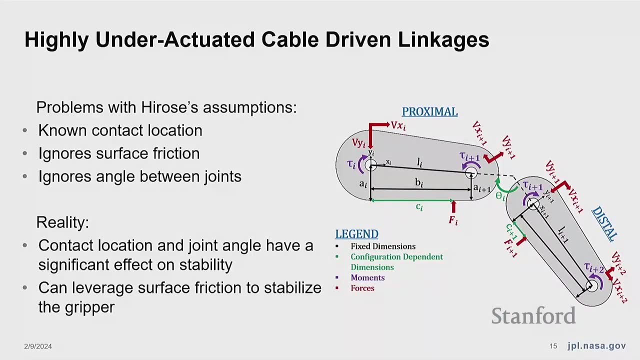 from a net negative to a net positive torque And it's going to rotate until it comes in contact with an object. If you remember that torque distribution that I mentioned earlier, there are a few assumptions that were made to get that torque profile and to guarantee that surface contact. 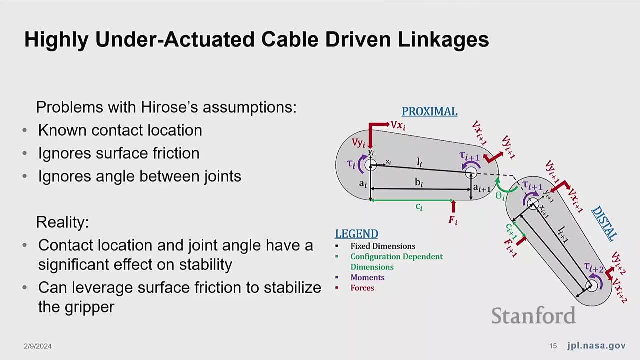 A few of those assumptions include a known contact location, ignoring surface friction and ignoring angles between joints. So it's a great set of math to derive that original equation. But as you add the real world and practical joints and it gets quite difficult to make an infinite number. 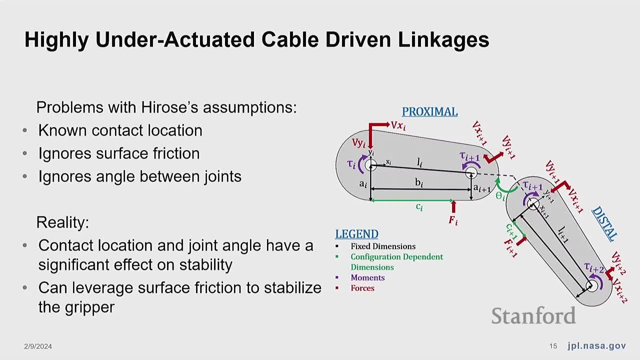 of joints. as you can all probably imagine, that some of that math does break down And basically this introduces a mathematical look at the stability of a gripper, Where stability is defined on its tendency to push itself off the surface, as you. 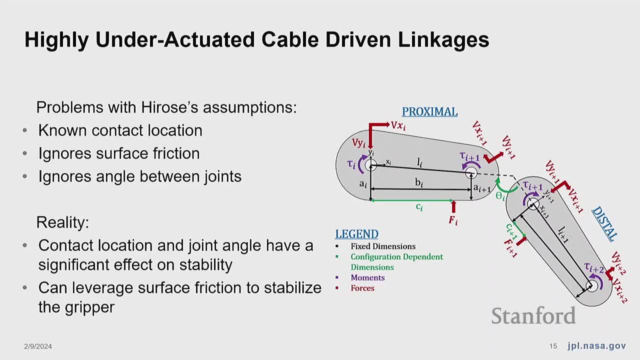 saw from that unsuccessful grasp in the previous figure. So in reality the contact location and joint angle have a significant impact on stability And the more joints you introduce it often becomes harder and harder to stabilize grasps on unknown objects, And part of that is simply due to the practical challenges. 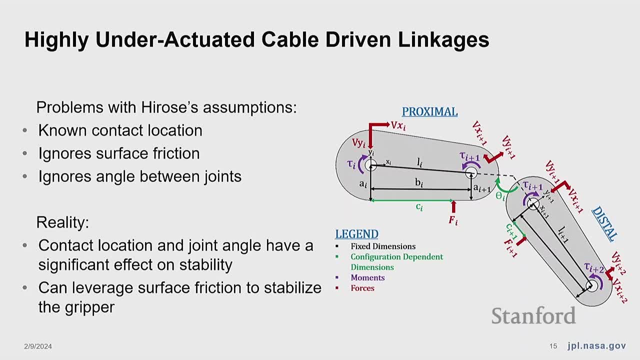 of packing And exponentially it becomes harder and harder to stabilize and expand. And so we're looking at this gripper as a way of exponentially scaling torque profile into a physical gripper with 10 plus joints. There's one big thing going in our favor. 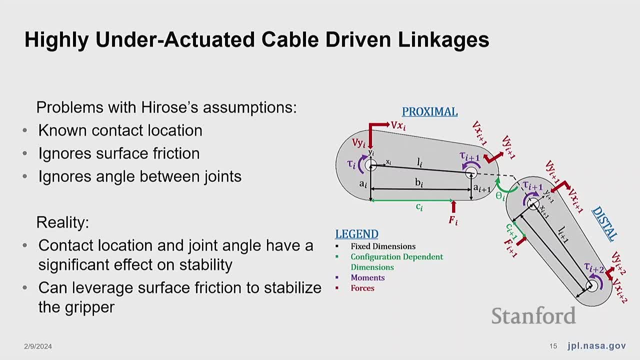 that already dovetailed really perfectly with the adhesive work that we were already pursuing. So again, we were looking at this gripper as a way to engage and contact a surface and then engage the gecko-inspired adhesives. So how can we wrap around large, arbitrary objects? 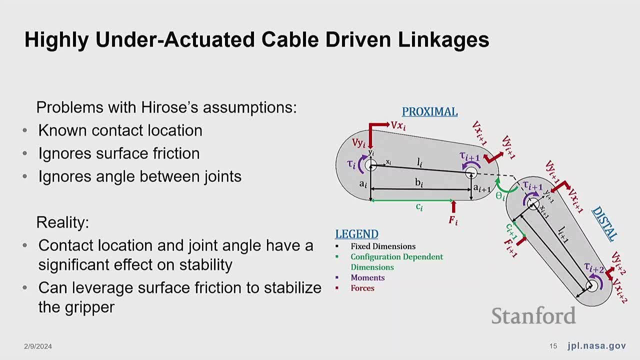 and then let the gecko-inspired adhesives do the work, And this led us to an interesting result, which is that the surface friction has a large and positive effect on stabilizing these grasps. So there's a lot more math, but for the sake of brevity, 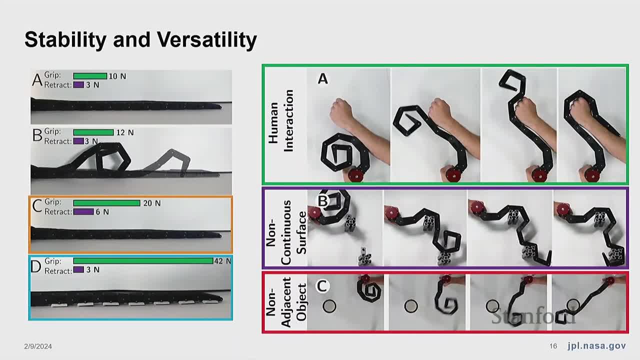 I at least just want to show the results today. Here you can see basically this behavior. on the top left here A gripper, right after the last link, has come in contact And you can see the force that we have in the grip and retract tendons. 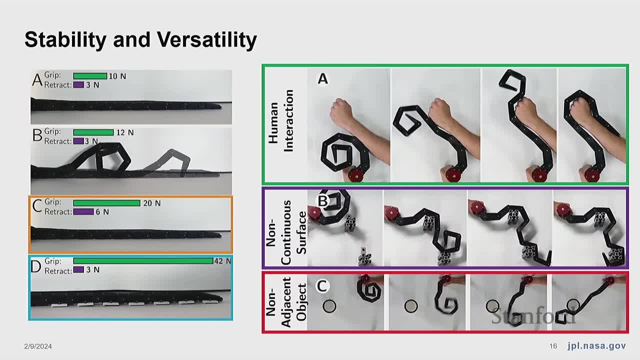 And you can see the force that we have in the grip and retract tendons. As we apply more force in the grip tendon, you see this loss of stability and the gripper pushes itself off this flat surface. There are two approaches that you can take. 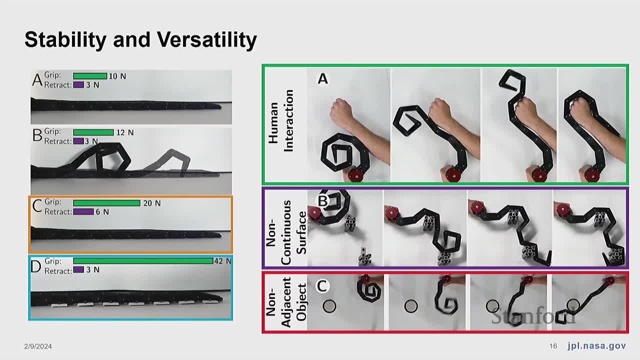 One is just purely mechanical: by scaling these forces but keeping the torque profile the same, You're able to maintain contact. The other is again by adding surface friction. So in the final figure here D, you see the impact of surface friction. 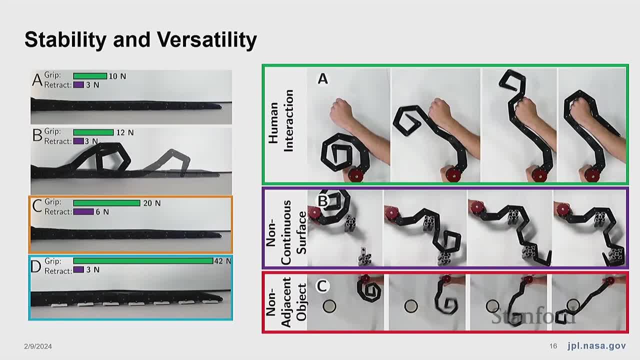 with a little bit of tension in the gripper. overall, It provides a lot of extra stability and we're able to engage and torque down onto the surface at a much higher level without losing contact. You also see some of the nice benefits of this style of gripper. 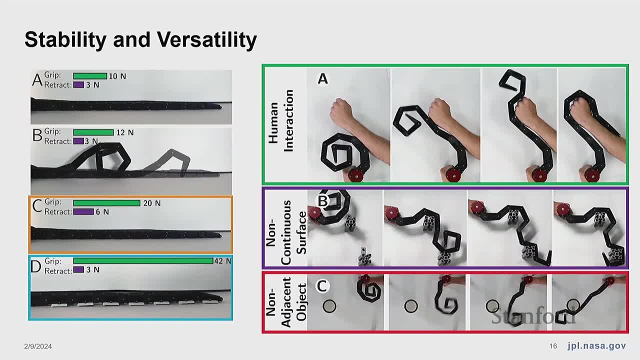 So because again, it is quite compliant, gentle, its torque into the surface is not particularly high. It can wrap around arbitrary shapes without damaging them. We show that on gripping an arm. It can potentially wrap around non-continuous surfaces or reach. 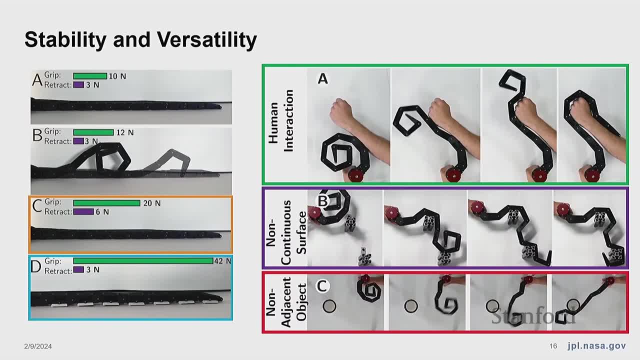 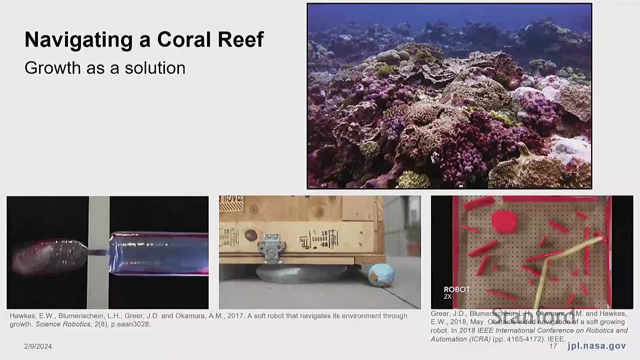 not adjacent objects. By exploiting dynamics and actuating quickly, you can actually choose whether or not you're going to do that sequential motion or engage multiple joints at a single time. I'm now going to take a little bit of a departure and start talking about coral reefs and growth. 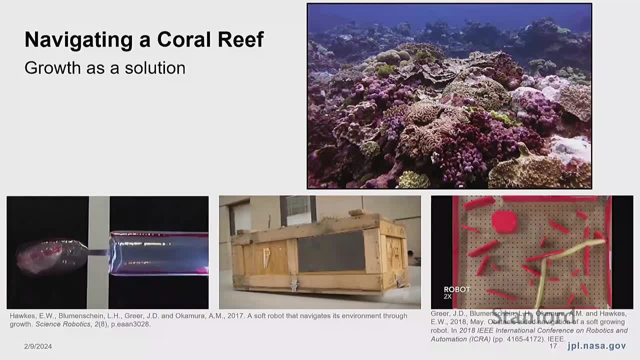 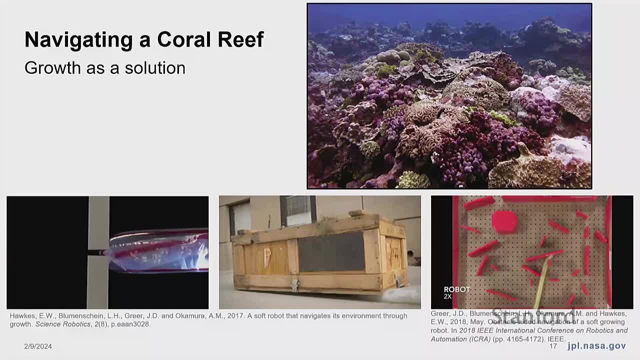 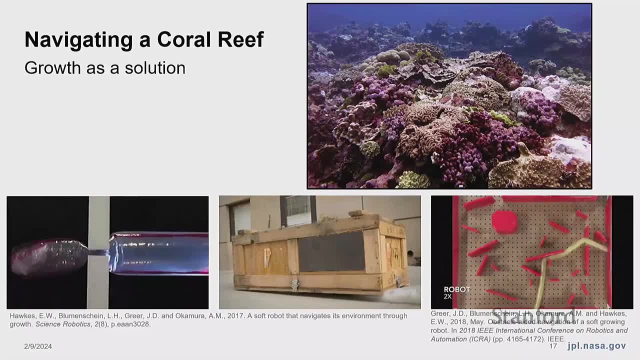 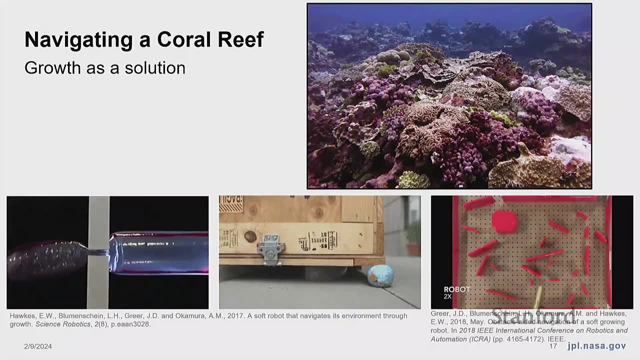 And I'll do a quick plug for Mother Nature here. Coral reefs are incredible and very worthy of fascination. They represent just 1% of the ocean's seafloor but are home to 25% of all marine life. Coral is alive and it's really a keystone for ocean ecology. 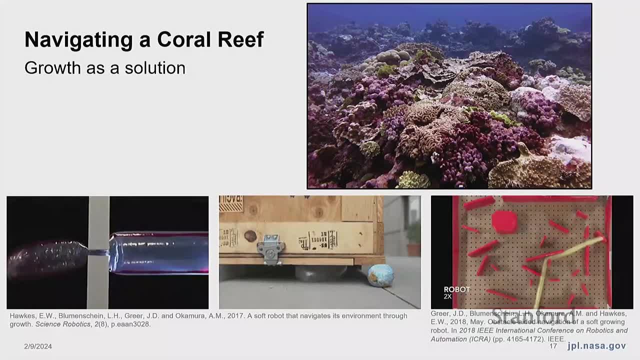 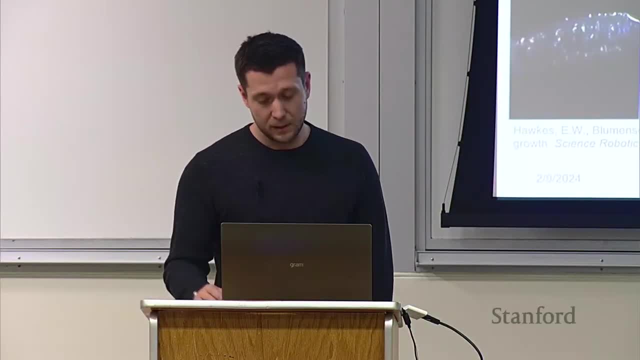 The sad reality is that there's also a race against time here, With coral reef collapse and bleaching events, So we not only want to prevent those, but we want to understand their mechanisms to help look at potential mitigations. However, exploring a coral reef is a non-trivial challenge. 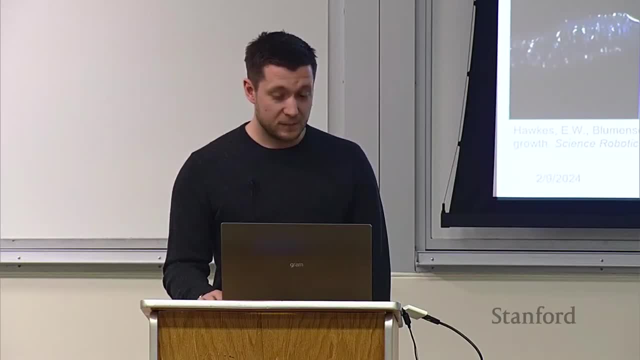 It is a complex, dense, unmapped three-dimensional space with tight cavities and abrasive- basically abrasive- properties. At a similar time, as we were starting to look at this exploration, some great, great research was coming out of Stanford here in Vine Robots. 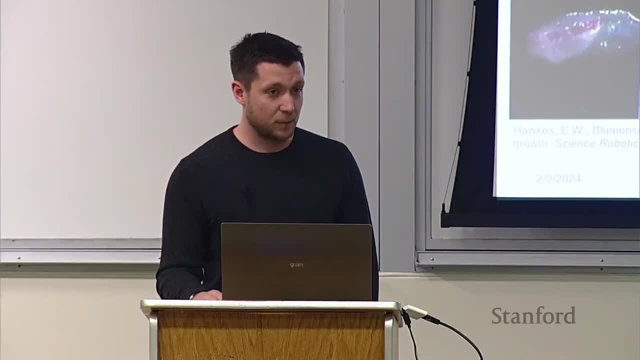 And we saw this as a potential solution for really a few key properties. First is a simple deployment mechanism, So you're just controlling the spool, the length of the spooled material, and then applying pressure, And then, additionally, it has an ability to squeeze itself. 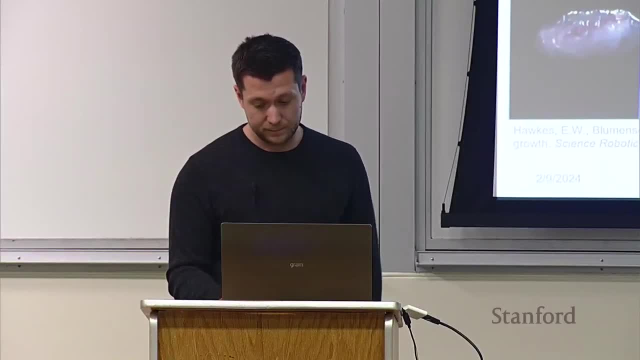 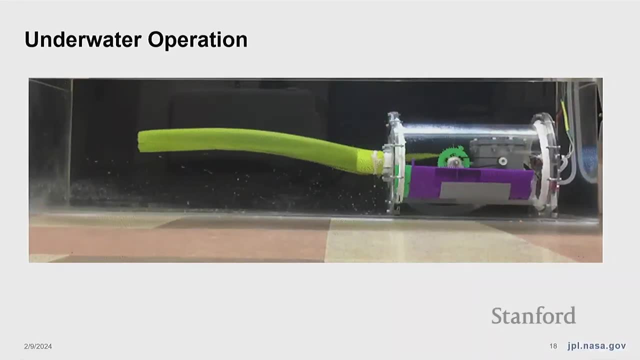 through tight spaces and self-navigate through cluttered terrain. So we basically built an underwater version. We did a few things: We have our motor and electronics inside of an internal waterproof housing And then we have this larger water-flooded housing where we're basically just pumping in ambient water. 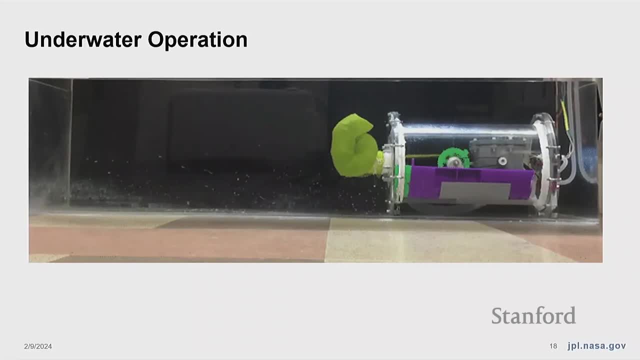 from around the environments. We're using the resources that are already there and leveraging that to drive the growth of the robot. You can see we maintain a very flexible, soft device. This is done at low pressures- less than 3 psi. You can see, even just sitting there. 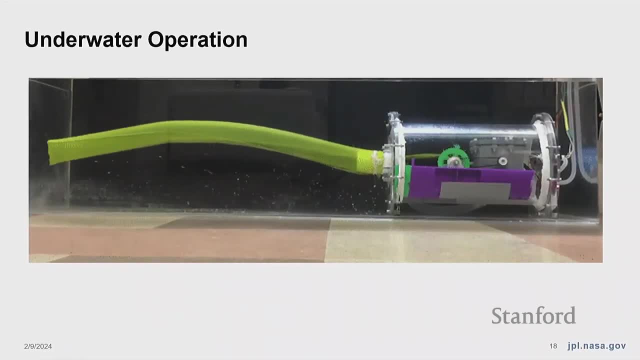 in the tank. it's basically deforming under the small currents that it created. You can also see it's too soft to basically support itself. Once you apply a retract load, it buckles and curls itself up. Of course, in free space this isn't so much of an issue. 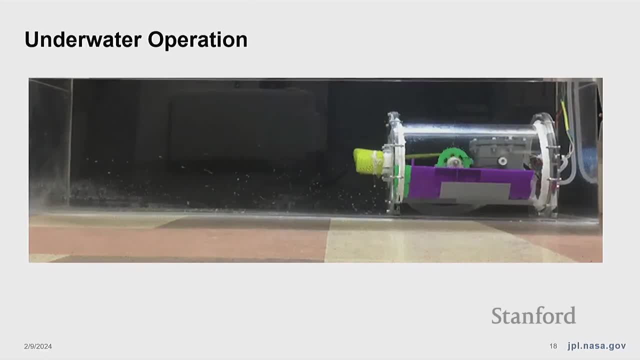 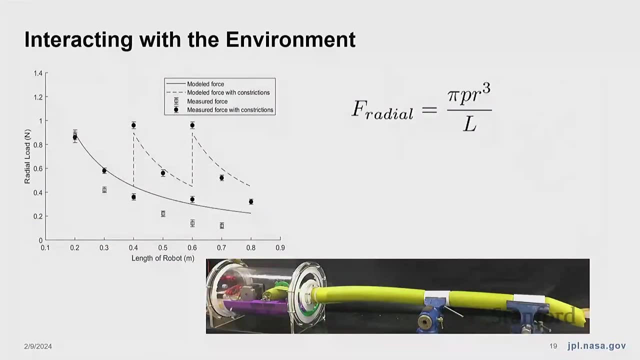 Because, once buckled, it'll then proceed with its retraction, And in a confined passageway this buckling doesn't occur, which led us to a few interesting small studies, which is that, again, the point of this work was to interact with its environment. 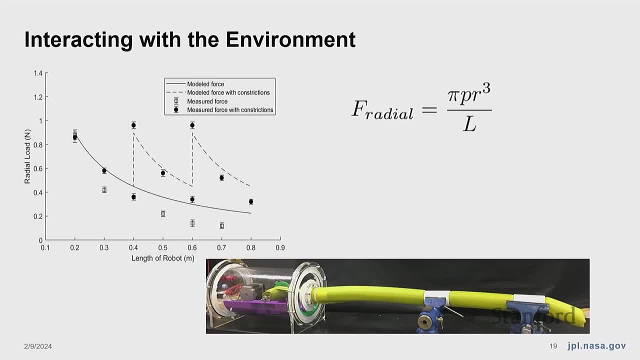 And what we find is, of course, that really what you're dealing with are inflatable beams, And they have two main modes of buckling: either through axial loads or radial loads. Both have a strong dependency on the length of the beam, But the overall length of the beam is not all that matters. 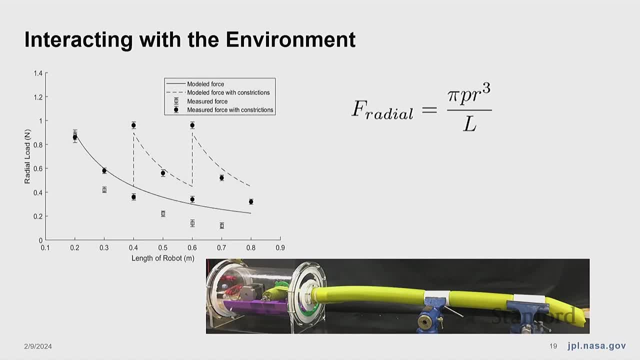 What really matters is the length of the beam since its last support or constraint. So again, this lends itself well to operation in cluttered and crowded environments. is that if you are interacting with the environment and that environment is causing to reinforce the structure of the robot itself? 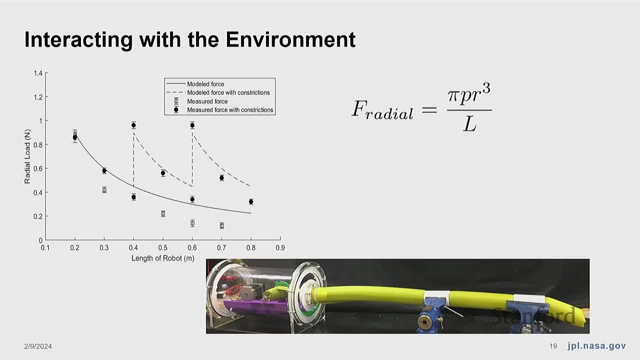 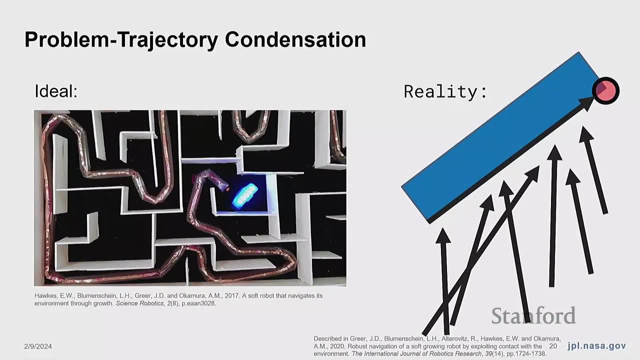 you can leverage that to support payloads over larger distances than you could in free space. There's one other problem as well, which is that in an ideal situation, you'd be able to navigate through a very cluttered space, But in reality, especially if you're doing this in open loop- 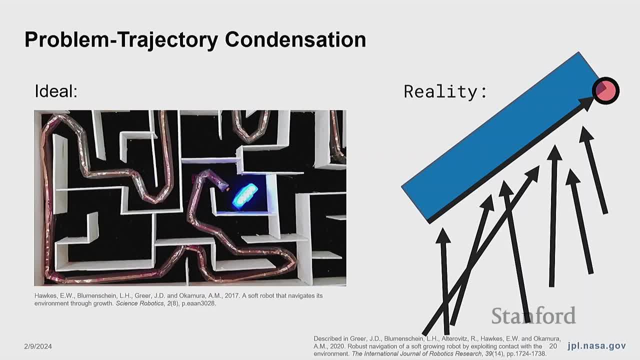 you have to face the challenge of trajectory condensation. So if you know what the environment looks like, you can either pre-program or control around obstacles. But especially again in open loop, you don't have that ability, So you're just going to run into obstacles. 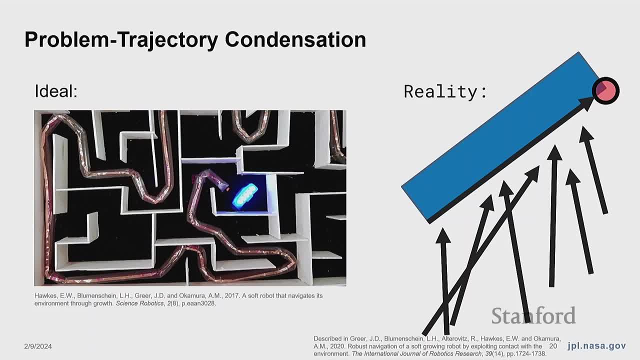 and basically grow along them until you depart. And what this does is it takes the infinite space of potential starting trajectories and condenses them all down to a single trajectory, leaving that obstacle. And this motivated us to look at how can you solve that problem and still potentially navigate a cluttered space. 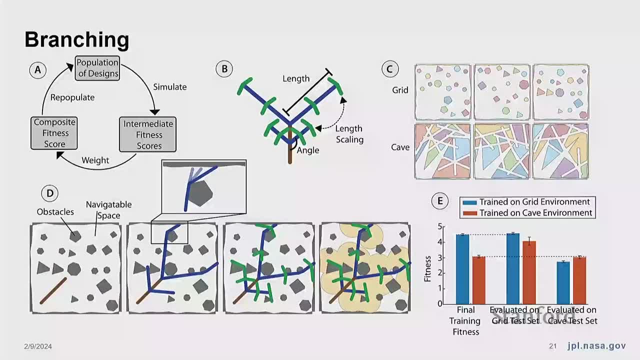 So I'm going to show you how to do that with Coral Reef Space in open loop. My work here coincided with the start of the pandemic, So again motivating flexibility and being able to pivot to a computational approach to this problem. So we looked at basically recursive branching. 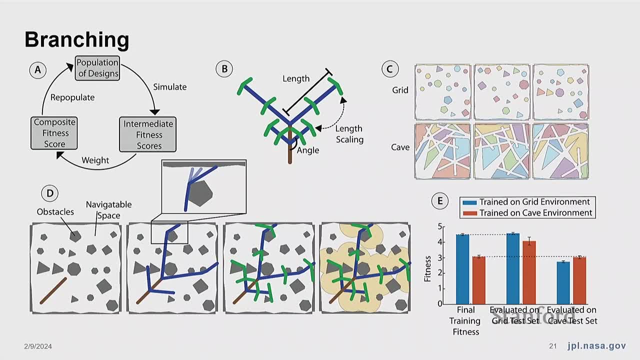 as a solution to this. So a path might be growing down a passageway that's going to end up in a dead end, But if you are deploying new material at new angles, you basically are able to avoid this trajectory condensation because you're not relying entirely on the obstacles. 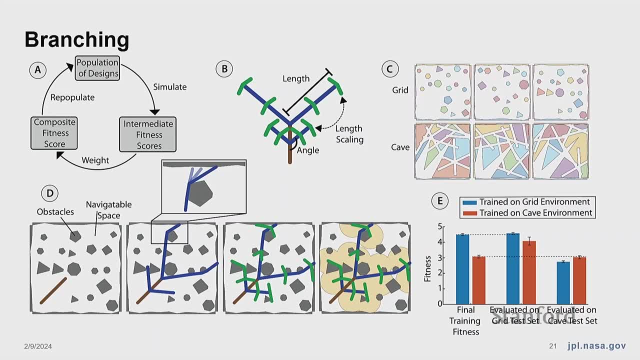 you've already hit. The other thing that looking at branching does is it gives us a richer design space so we actually can attempt to optimize and improve our ability to explore an environment during the design phase, which again saves important resources and effort when in the field. 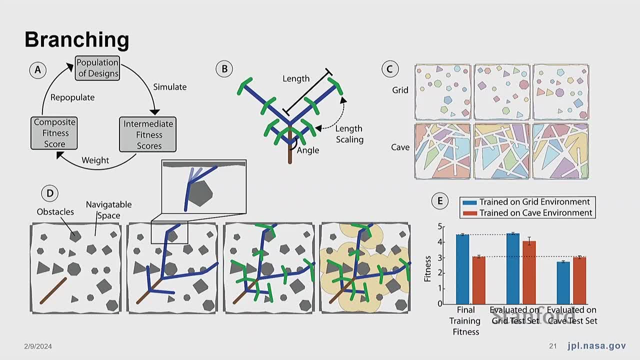 Because that operations phase, if you're underwater and have a diver on a fixed supply of air, becomes a much more pressure, It's not just a resource. So to do this and try to improve our performance on unknown environments, we looked at 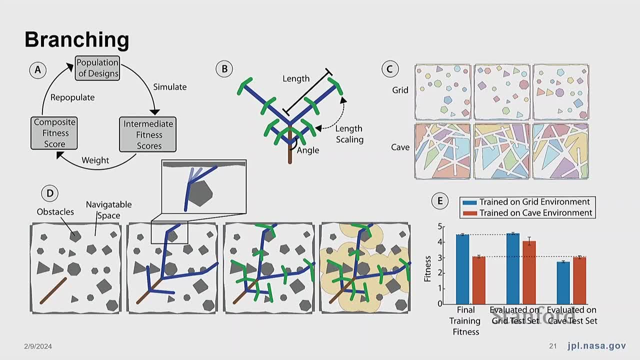 can you train on known examples and then use that, basically learn something fundamental about the environment, improve your performance and then see that performance improvement hold steady even when you do go to deploy in the field. Towards that, we basically set two different. 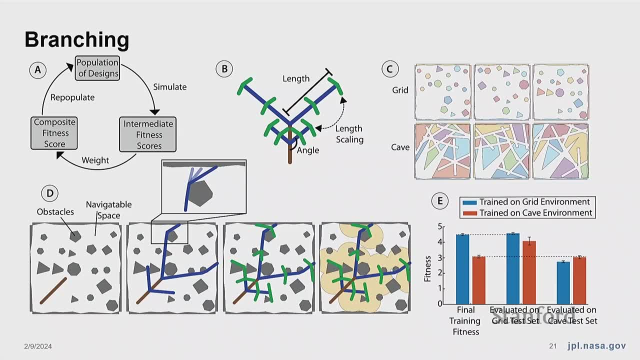 simulated environments, a grid and a cave, example environment, And you do see, basically, specialization of these optimized designs on each environment. So they were trained on a training set and then they carry over that specialization and show each their own, each design that was trained on one environment. then 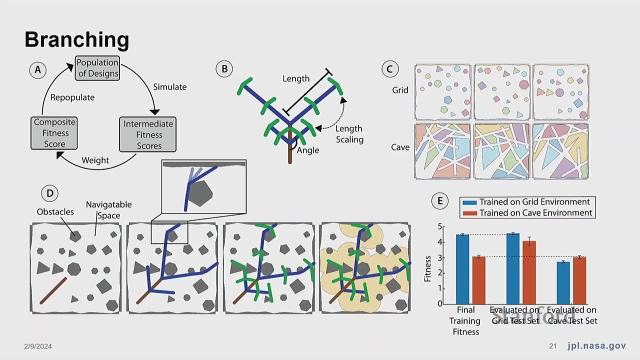 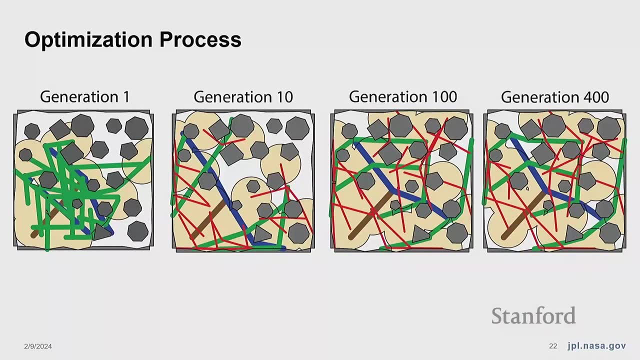 performs the best on the same training evaluation environment. Here you can see just a visualization of the optimization process. So this is generation 1,, 10,, 100, and 400 of an evolutionary algorithm. We were awarded coverage. We basically treated this as a sensor distribution problem. 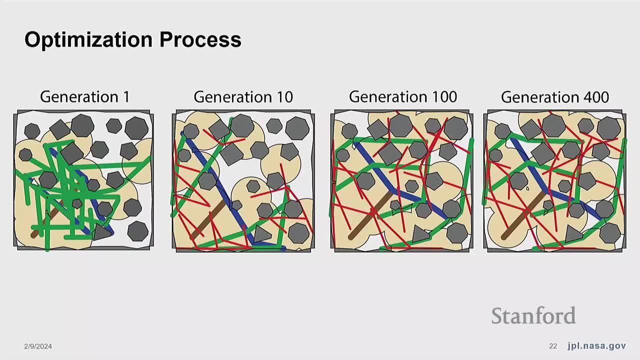 So we wanted each end of the robot to end up in as unique a location as possible to try to cover the entire space while penalizing overall length of the robots. We wanted to do a material minimization as a here is stick for simplicity, And here you just see, basically snapshots. 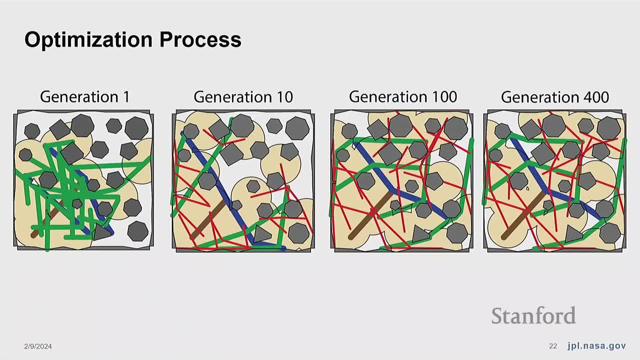 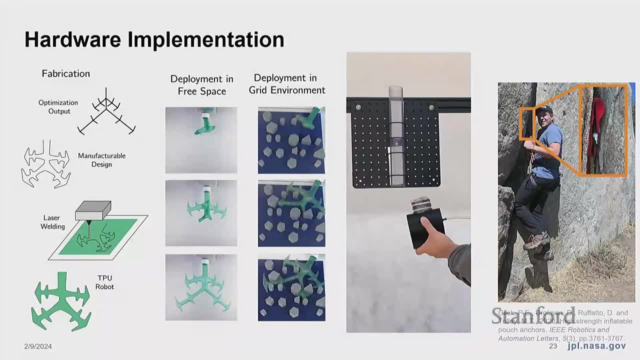 of the design across generations, all plotted on the same evaluation map. Towards the end of this project, we were able to get back in the lab and do a little bit of hardware implementation. We worked on fabricating. How do you actually take these optimized designs? 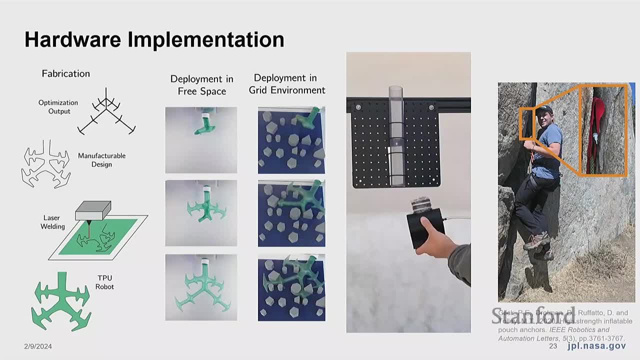 and then turn them into a manufacturable design. I will say that prototyping and building branching fine robots remains to be a challenge. If anyone solves it, please do let me know. We did get some progress. had a lot of fun doing it. 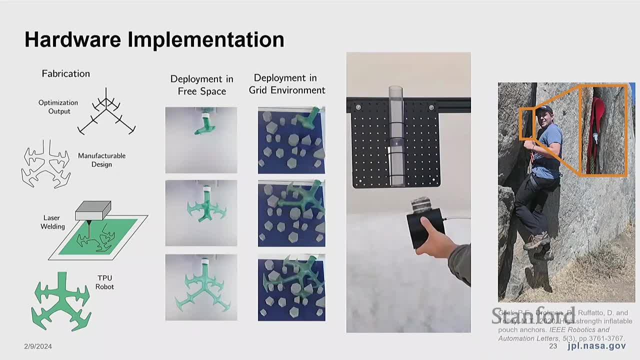 But it is difficult just dealing with that amount of internal friction and material transfer, especially over long distances. We also looked at a little bit of a parallel property. This is basically if you're deploying material into an environment and especially with the confirmation that you get from pressure and expanding. 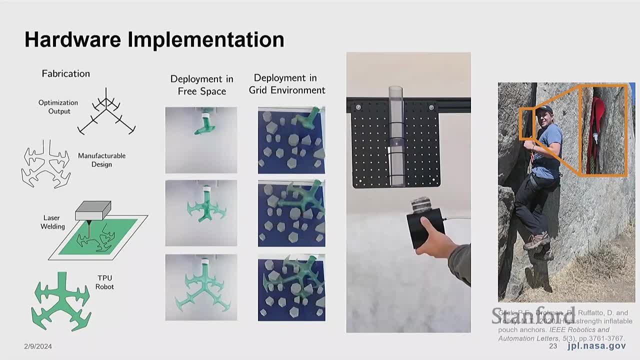 outwards into this constrained environment. it almost presents a new approach to gripping through anchoring. So here you can see basically a vine robot growing into a constrained space. It works best if you're in a tube that matches the diameter, But even again, a cluttered space with branching. 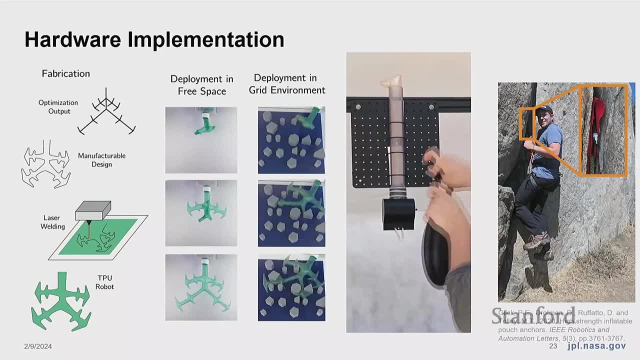 shows a similar property where you're able to wrap and deploy around objects And despite a very low pressure and growth, just again that large amount of friction. 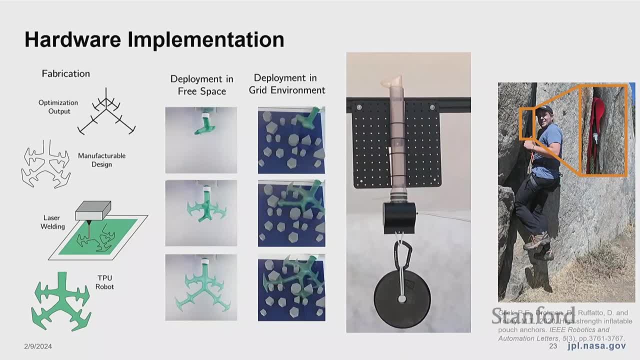 over a large area. it's much more about what you can do to deploy the system rather than the strength that it needs to do that, And we took this and further exploited it, making an anchor- a small pouch anchor- that you can use to actually well. 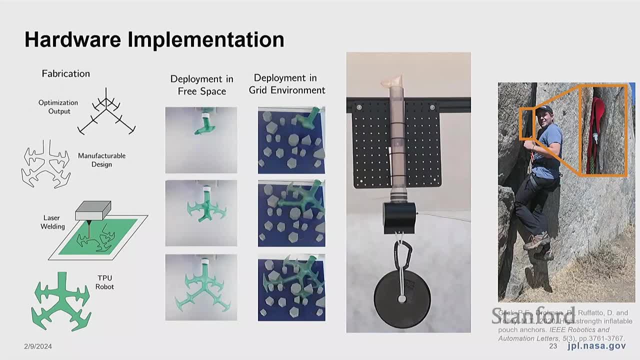 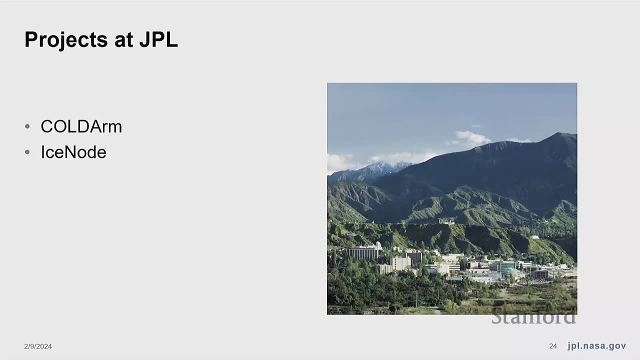 don't use this to rock climb, But we show at least it can support a human off a very small initial volume of air. Now I'm going to switch gears a little bit and talk about two of my projects at JPL. you're gonna see that there's a similar trend here, focusing on simplicity. 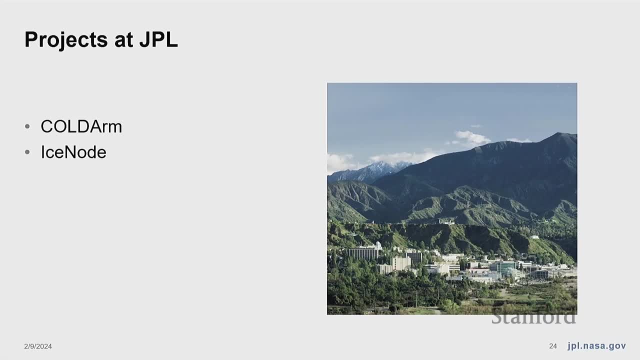 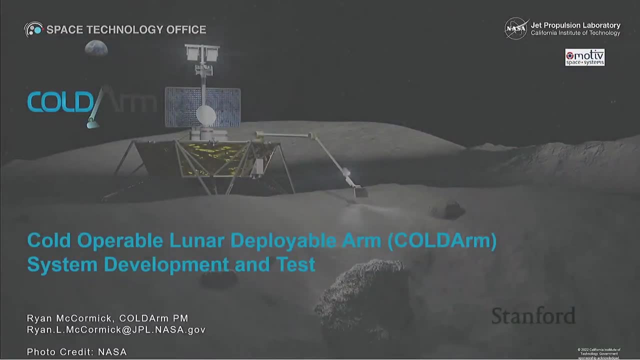 for these extreme environments. They have a little bit different of a flavor and they're both focused on really quite cold environments. So the first is Coldarm. This is a project in partnership with Motive Space Systems and led by Ryan McCormick at JPL, but this is motivated really by the thermal power consumption. 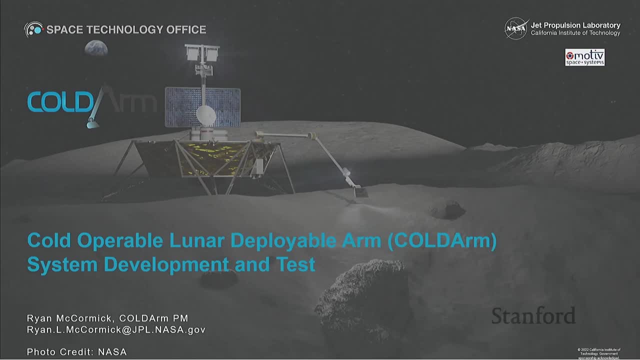 that it takes to maintain operations in cold environments. So if you have robotic arms that go to cryogenic environments, which is common, you know Mars at night is a balmy minus 90 Celsius. The moon gets way colder, down to below minus 150 Celsius, and at those temperatures you have to commit a 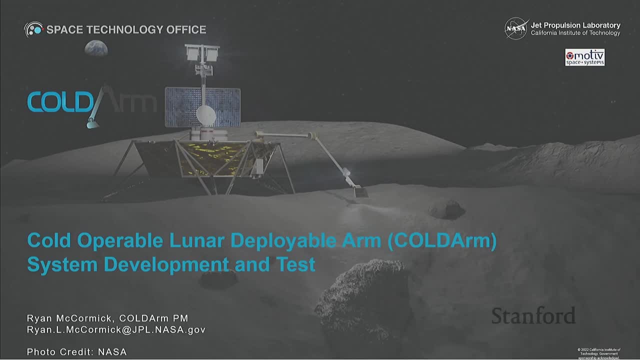 lot of power just to surviving the environment. but even when it's slightly better than that, you still have to expand the temperature a little bit. So that's one of the things that we're working on right now. So that's one of the things that we're working on right now. 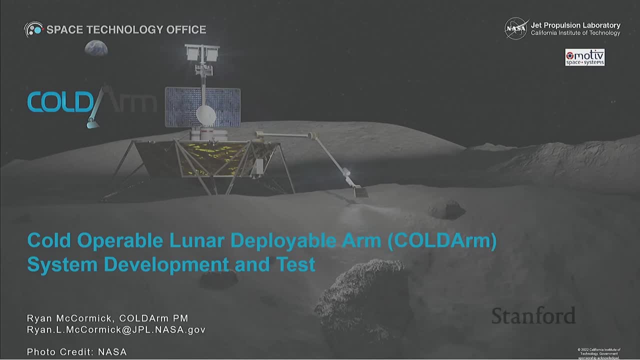 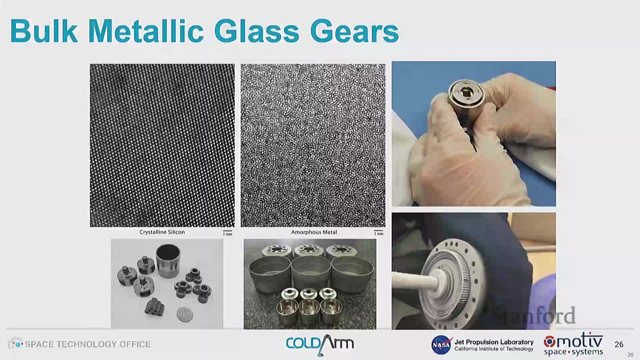 So that's one of the things that we're working on right now. You don't have to spend a lot of power just to heat your actuators. keep lubricants moving, things like that- So similar to a lot of the Gecko inspired adhesive. 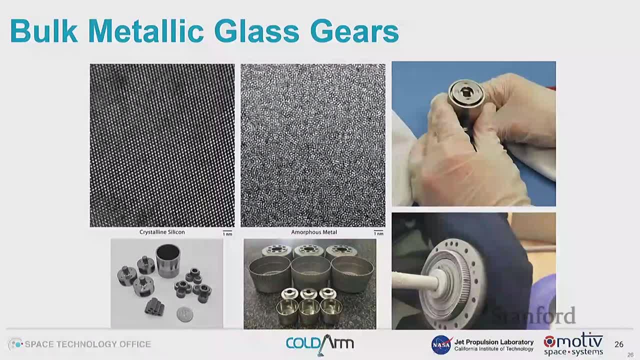 projects. this started as a material science and really more fundamental approach, looking at bulk metallic glasses. So you know, glasses we think of normally having a crystalline structure, but if you use amorphous metals which you can get through certain heat treatments and processes, they're actually 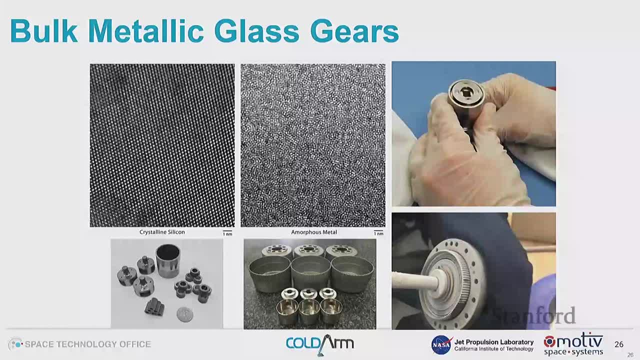 able to maintain their elasticity and flexibility down to very cold temperatures, which of course has advantages for space where we're operating at those cold temperatures. There's been a lot of great fundamental research on how do you take these kinds of materials and actually work with them. 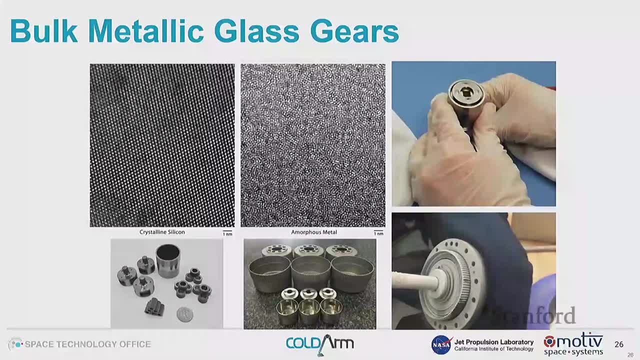 and turn them into useful parts. A lot of the things we like to do to make parts, like forming them, extruding them, molding them, all involve heat. even cutting right, just the friction of that can generate heat, and because the heat 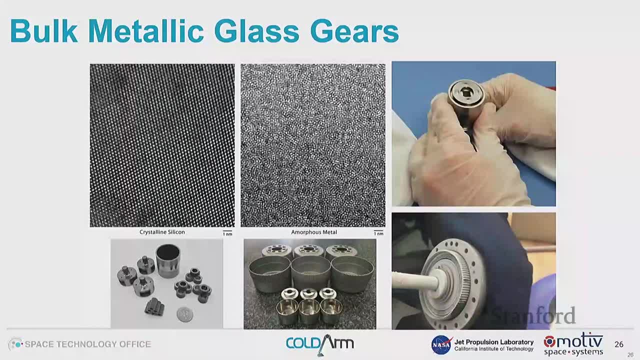 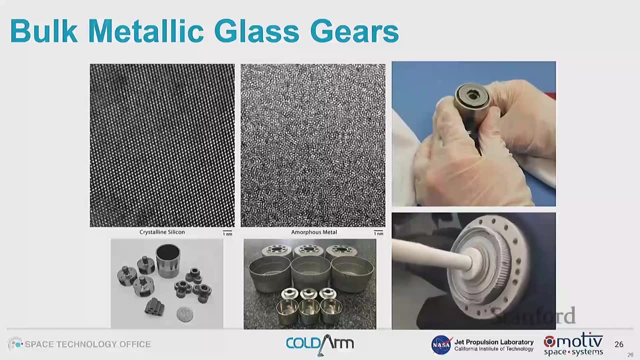 that you generate during manufacturing really impacts this material structure. there's a lot of interesting challenges here. You can see this is a basically gear set for a small motor, and then here's an entire harmonic gearbox that's been previously submerged in a liquid nitrogen bath. so down at 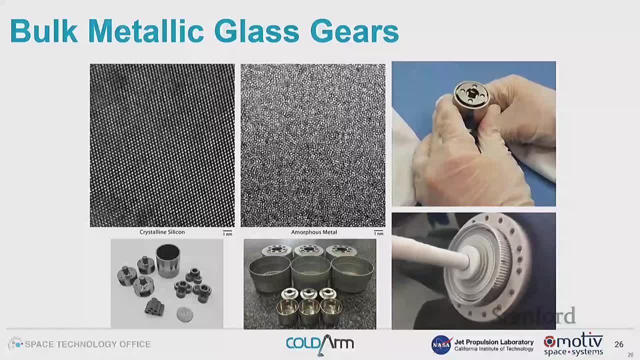 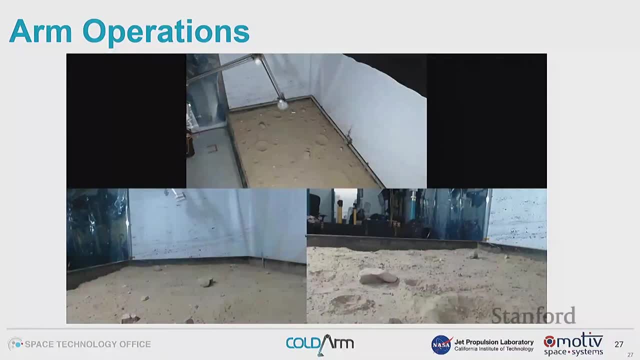 minus 180, still happily spinning and flexing during heat. Down that cold. Here you can see our robotic arm in a simulated test bed. so basically, this is a. is the video stuttering? Well, hopefully that resolves itself. The arm was smoother than the video. I'll 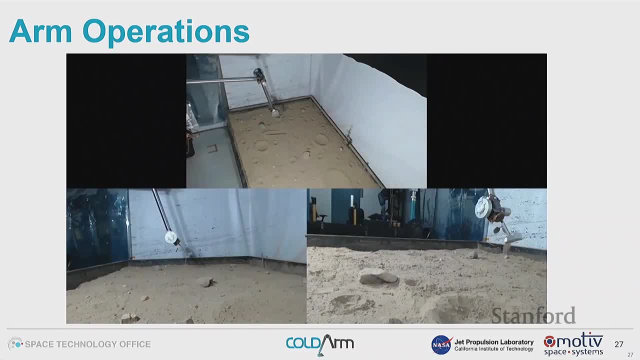 tell you that much, but there's two points that I want to bring up here. First is the challenge of designing things for space and using the materials, having to do much more custom and having to build things from scratch when you can't go to a commercial company and buy an arm off the shelf And then using 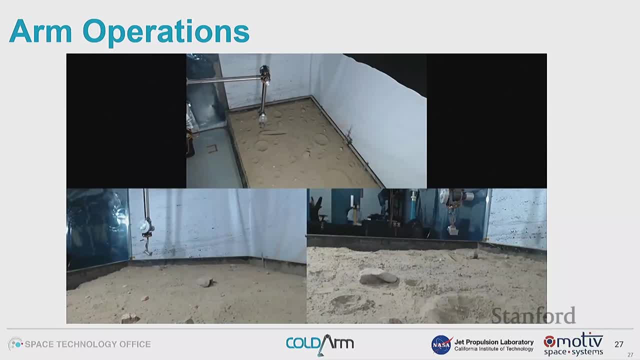 your ground data station, as you would if you didn't have a great telecommunication link. The other thing that I like to highlight here is the ingenuity of scientists themselves. so again, the motivation, the need to be as for a lot of these operations in extreme environments. 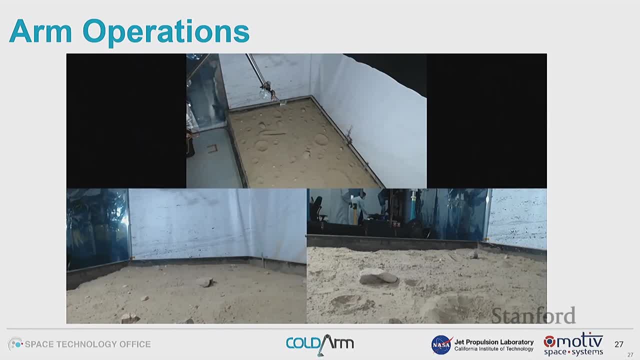 is the science that you can achieve here, And we'll see if, Oh yeah, there's the arm working a little bit better or the video working a little bit better. So you can see here it's a pretty simple end effector. 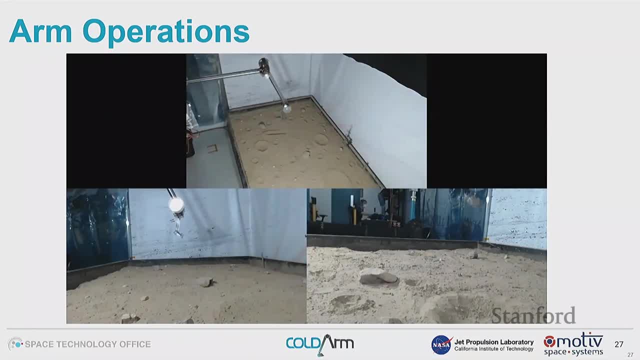 It's basically a scoop and a pressure plate, But even through that we're able to collect valuable data. So by scooping and piling that regolith into the same location you can actually measure the angle of repose. Similarly, by just pushing into the surface. 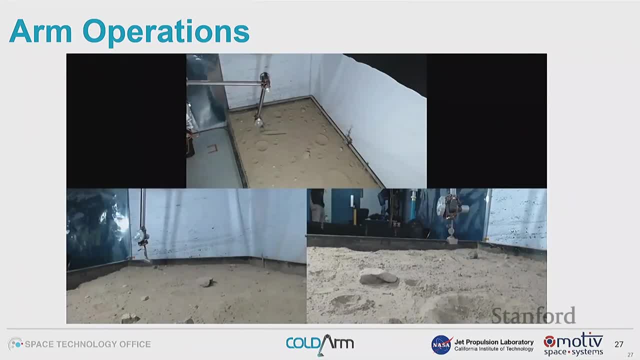 with a known load that we have through our forced torque sensor and feedback, you're able to learn a lot about the properties of regolith. So I really just want to highlight if you're able to get to these extreme environments, even small actions and small studies. 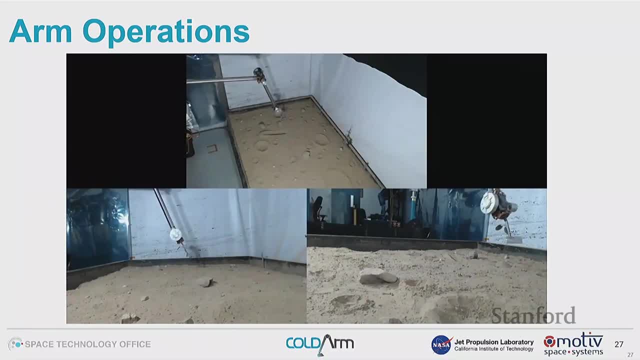 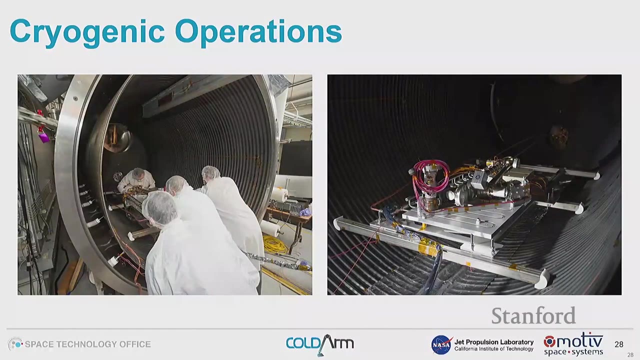 you're able to still back out a tremendous amount of information, just simply because getting there in the first place can be quite difficult. Oh, that was two slides. Here you can see us. This was a test we just completed earlier this month, so I don't have the videos from it yet. 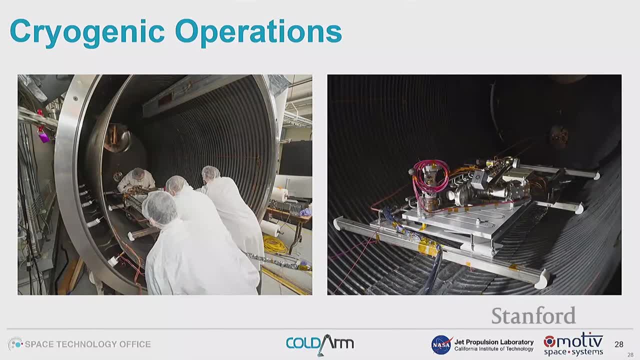 But we do have- at least our setup- pictures of us loading the arm into a seven-foot thermal vacuum chamber down at JPL. Yeah, so you know. the reality is, of course, that testing is a huge part of anything we do before we send it to space. 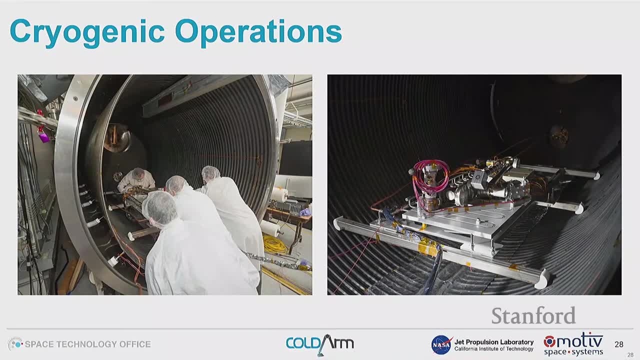 You really do want to burn down as much of the risk and uncertainty as you can before you commit to sending something out that you won't be able to service and maintenance. This test did complete successfully, so we showed the elbow joint, which was one of these amorphous. 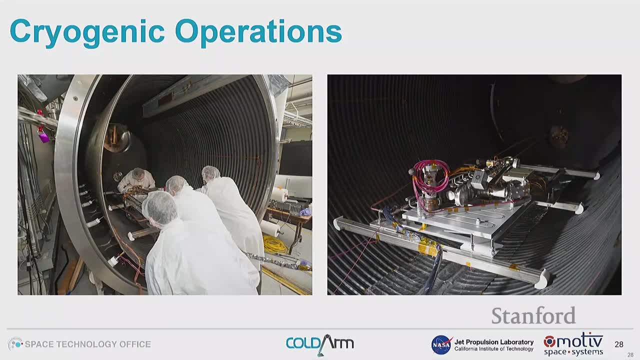 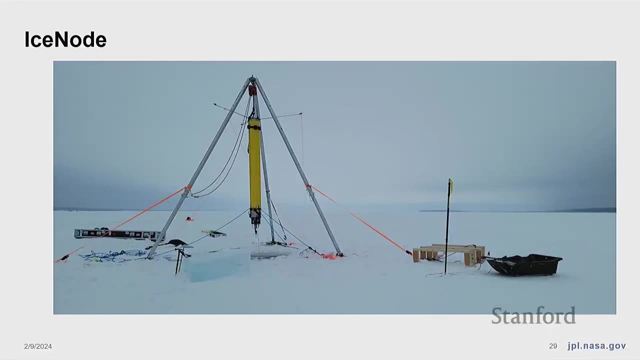 metal bulk, metallic glass joints operating down to minus 150 Celsius, which to my knowledge is the coldest robotic arm operations that I've heard of. And with that I'm going to turn to one of my final projects here. 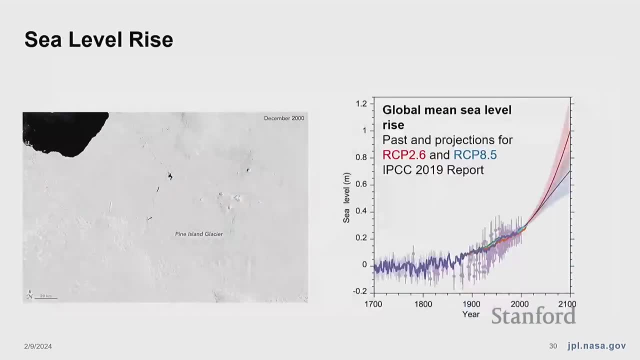 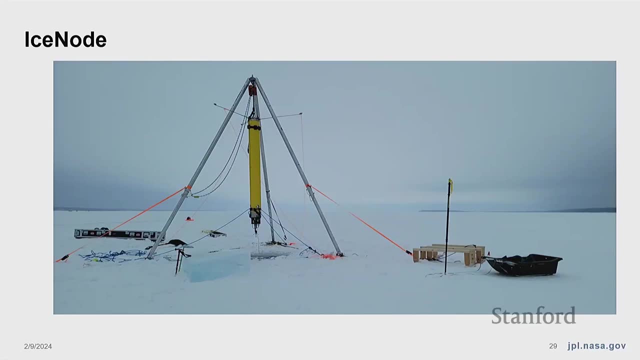 which is called IceNode. So IceNode is a. actually I'll stay here for a little bit. IceNode is a fairly large drifting robotic vehicle. It's focused on being able to drift underneath ice shelves over long distances and for long periods of time. 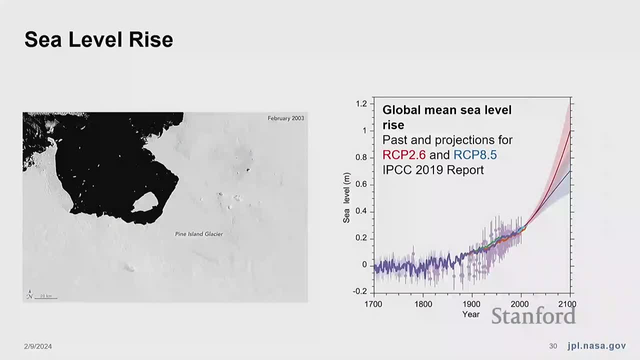 And you might ask: why are we trying to do that? The real answer is that we're trying to reduce the uncertainty on sea level levels. We're trying to reduce the uncertainty on global mean sea level rise projections. So again, I'm going to go into a little bit. 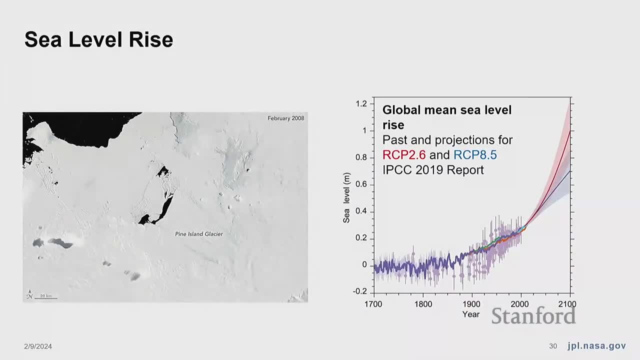 of the science motivation of this here. But there are these very large error bars on predicted global mean sea level rise And a lot of that uncertainty comes from, basically, glaciers that are sitting on top of Greenland and especially Antarctica. So these glaciers are all basically ice. 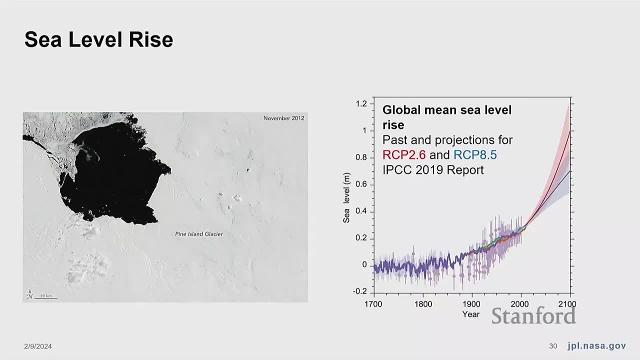 that's locked above sea level, currently happily sitting in ice form that is slowly flowing out to sea, And then, once it hits the water, the glaciers are going to go down. And then, once it hits the water, it raises sea level. 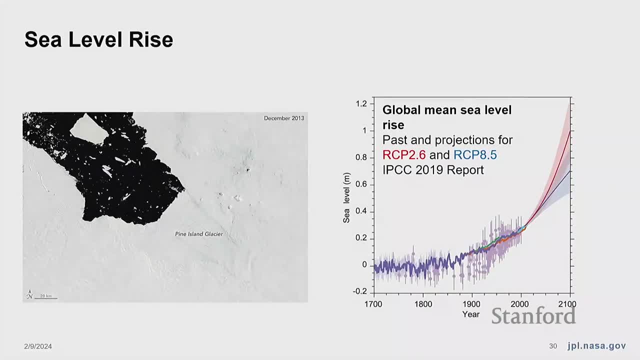 And the reason that it's flowing is because, at these size scales, ice is not really like a solid, It's almost like a honey material. It's this slow, viscoelastic process flowing into the water And this process is slowed by these basically ice shelves. 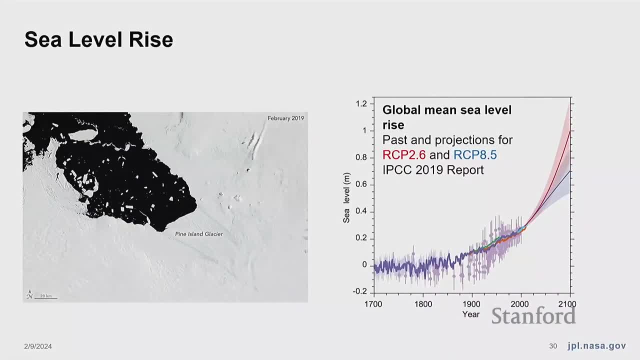 that effectively buttress these glaciers and slow that flow of ice out into the water. These ice shelves are experiencing rapid, rapid, rapid, rapid, rapid, rapid deterioration and collapse And we have a. you know there's a lot of great people studying this. 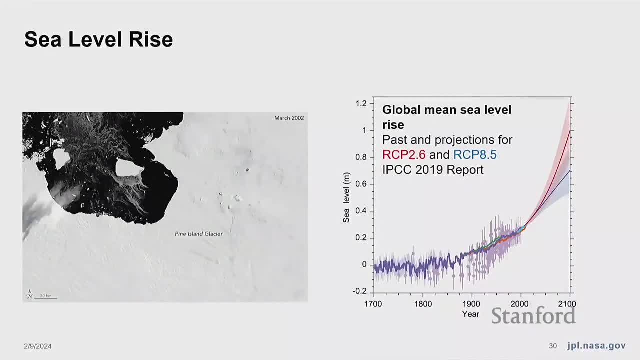 but still a poor understanding of some of the mechanisms and mechanics of these collapses, And the reason for that is because studying them is incredibly difficult, potentially over very dangerous places. You know you don't want to be out there when these sea ice shelves. 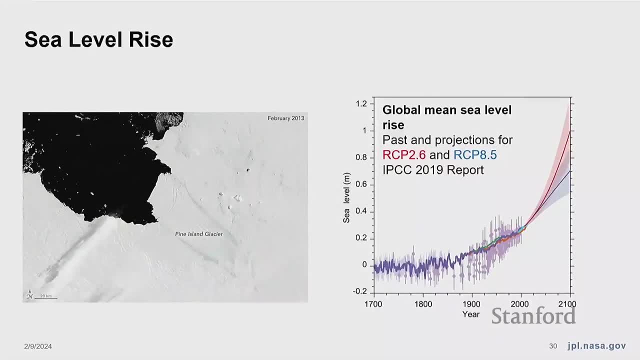 are basically breaking up or moving. So, again, it's a challenge to be able to understand what's happening in these again unstable, extremely cold, remote locations And, additionally, some of the best data where the melt is actually occurring is not on top of the ice. 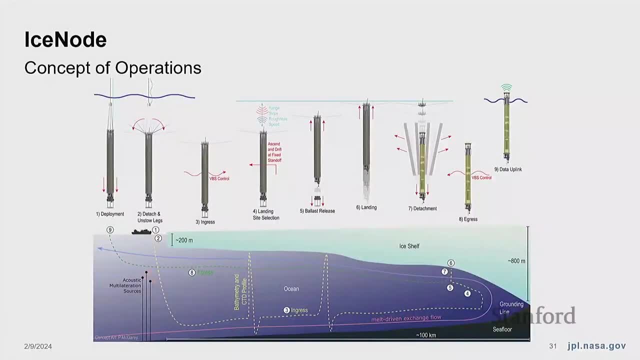 It's underneath the ice because you have this warm water coming from underneath. But, again, focusing on simplicity, and how do you take the things that are there in the environment and use that to inform the design, That warm water that's causing this melt? 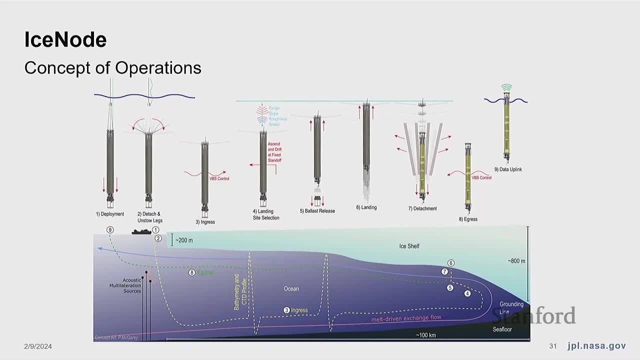 is actually very efficient in terms of energy. You basically have this current flow where you have warm water coming in along the sea floor and then it basically is rising up, contacting the ice shelf. that is causing some melt, so the water temperature is then cool and then flow back out to sea. 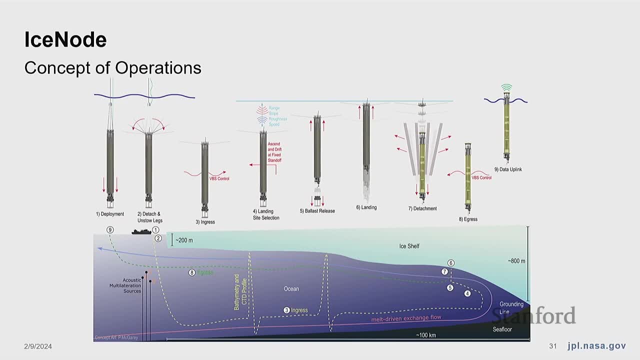 And so that gives us an approach to effectively drift in. So we have again, as I mentioned, the only real continuous degree of freedom that we have of these systems. We have a small oil-filled bladder that we can use to either pump oil. 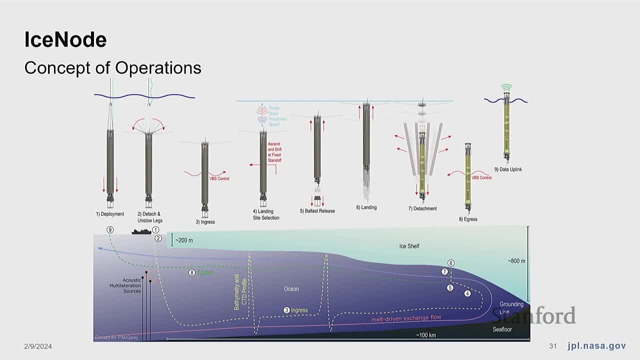 inside or outside of the vehicle, thereby changing its volume and changing whether or not we're going to sink or rise. Using that, we can pair with projections and estimates of these three-dimensional currents, basically pick what height or altitude we want to be at. 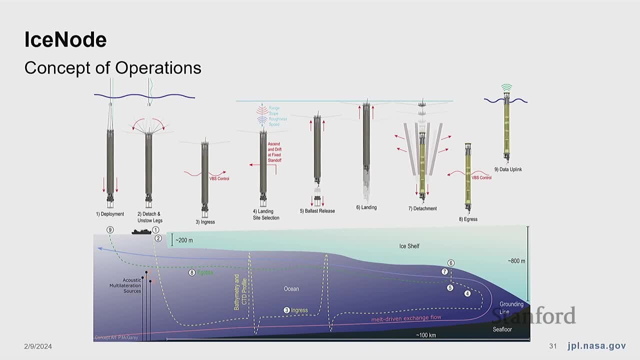 ride particular currents in and try to distribute a fleet of ice nodes across an ice shelf. Once we reach the point that we want to deploy, we have a heavy ballast that we can drop. This is a pyrotechnically severed device and we drop this ballast. 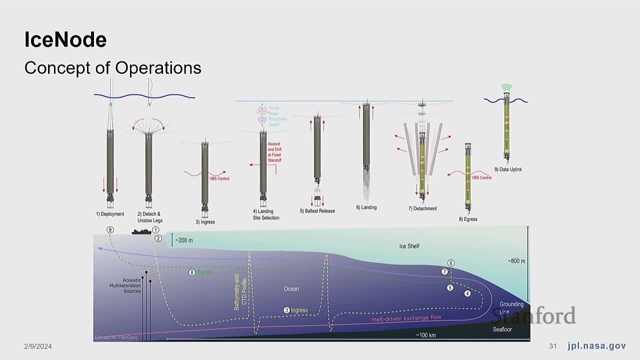 which then shoots the vehicle up to land on the ice. We have these three compliant arms that basically hold us steady. This is important because the science measurements that we're taking are measuring- it's basically sensing- these small turbulent eddies, so as the ice is melting. 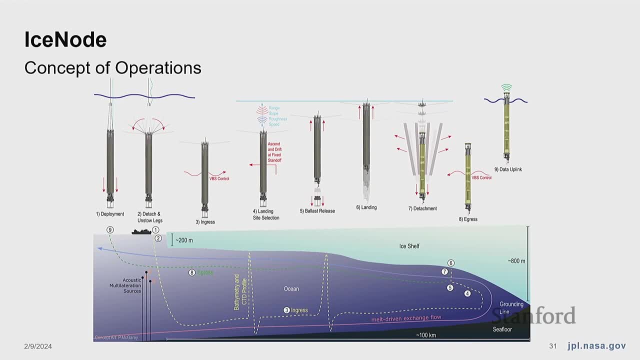 you have cold water flowing down into these small eddies and you need to be very still to be able to actually sense those After a period of months, then it's hard to transmit data from beneath a lot of ice. The approach there is then. 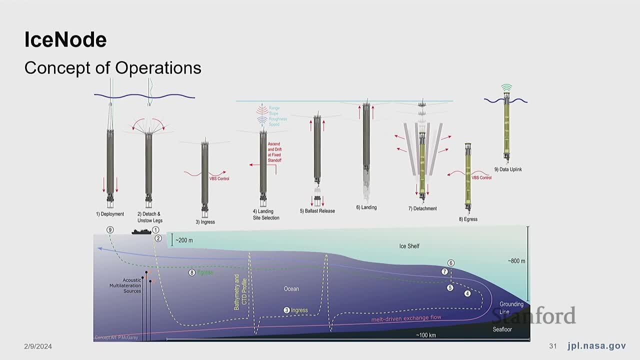 to be able to detach from those legs and from an extra set of flotation, return to a state of neutral buoyancy and then, when we're at that neutral buoyancy again, we can control whether we're positive or negative through that variable buoyancy engine. 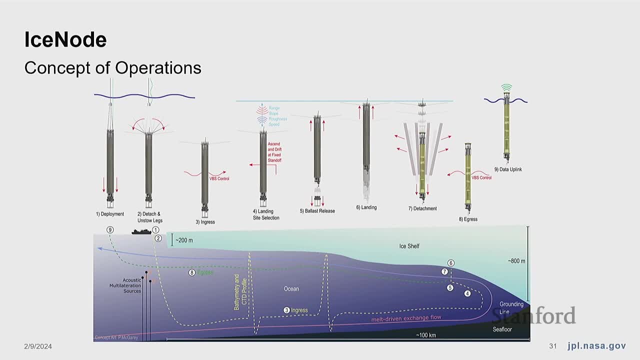 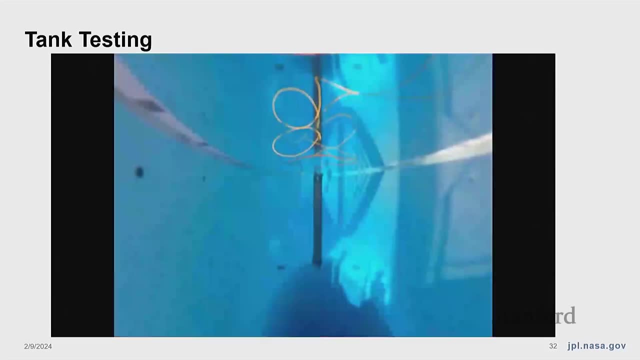 Then, once we're back out, we can take the open water and return the data. Here you can see some of the system functions in a tank test that we did in San Diego. In this case, our vehicle was better than the camera used to take the video. 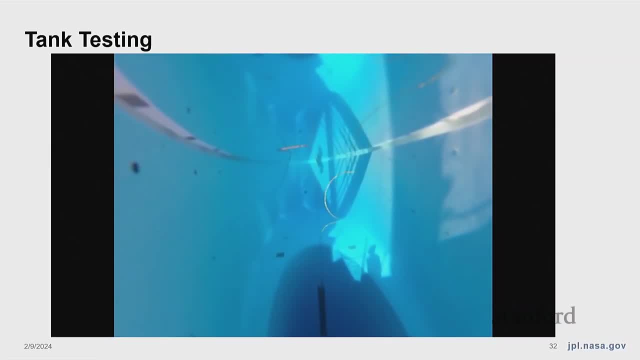 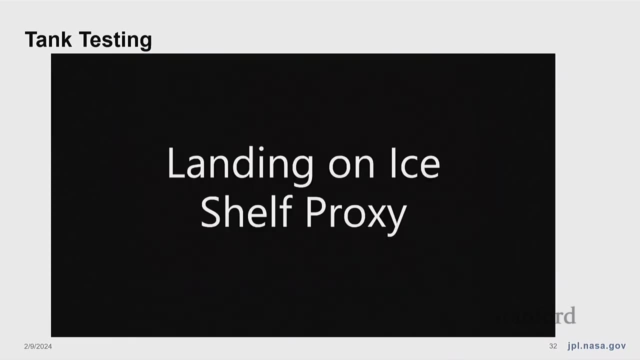 Here we're just checking out, going through a range of set points for depth control. Next you're going to see us landing on our ice shelf. It is, of course, difficult to find natural ice in San Diego, especially in the summer, so we had to use a plywood proxy. 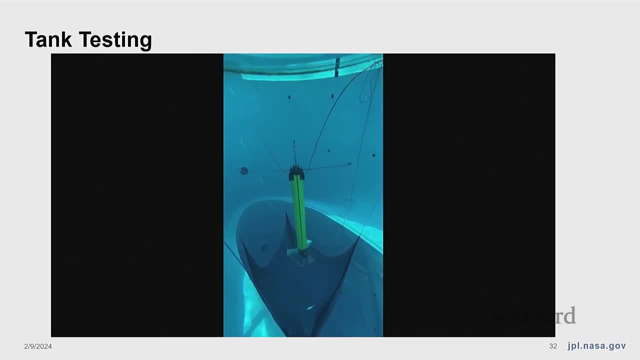 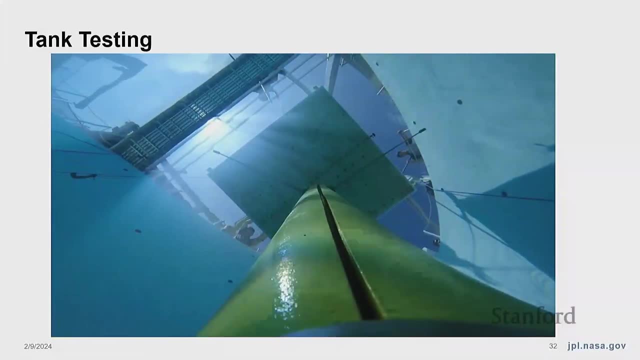 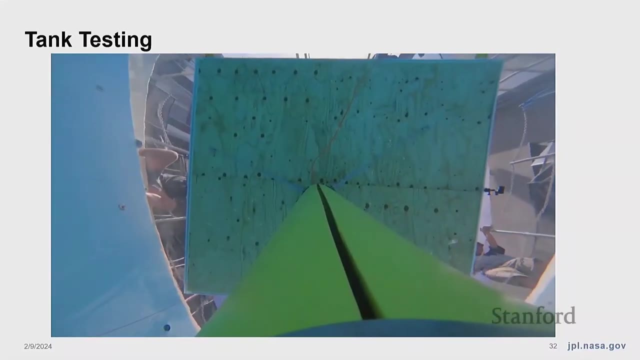 Here you see us basically severing this ballast and then launching up and landing on the ice. We have again these compliant legs that are spring-loaded to be able to react and absorb any of the differences in ice that we see. Then there's one more view. 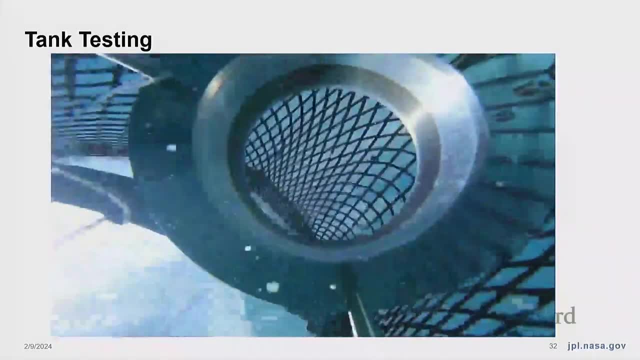 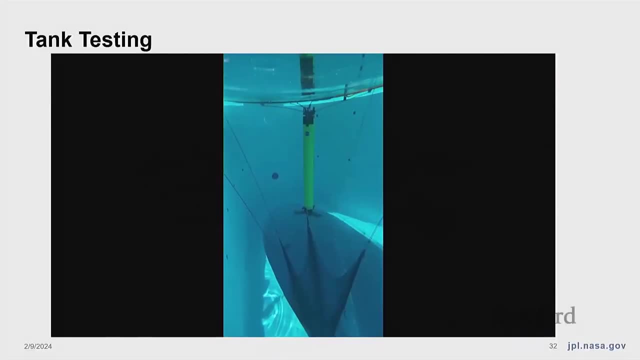 that'll show basically the weight clearing the instrument panel on the bottom. Then, finally, as I mentioned, we have a detachment at the end. This serves two purposes. First is, as I mentioned, we need to be able to return to neutral buoyancy. 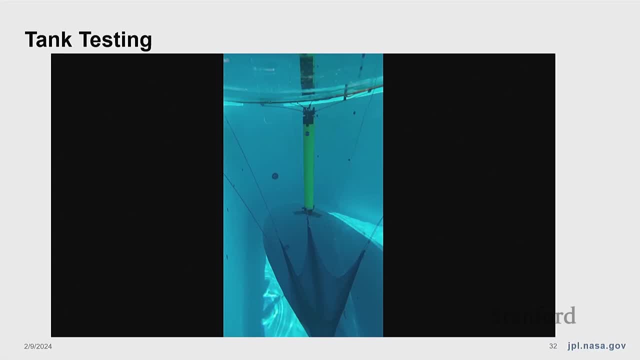 so we have a lot of buoyancy that we need to get rid of. Then the second is actually that there's a risk here of being able to melt the vehicle somewhat up into the ice. As I mentioned, there's warm water that's causing the melting flowing. 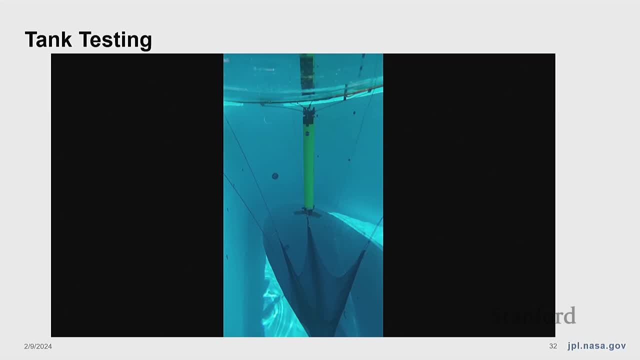 and if that flows over the vehicle, the vehicle might heat up just ever so slightly, leading to the ice that it's landed on. Then, even no matter what steps we take to minimize thermal conductivity, if the vehicle is warmer than the ice it's going to want to. 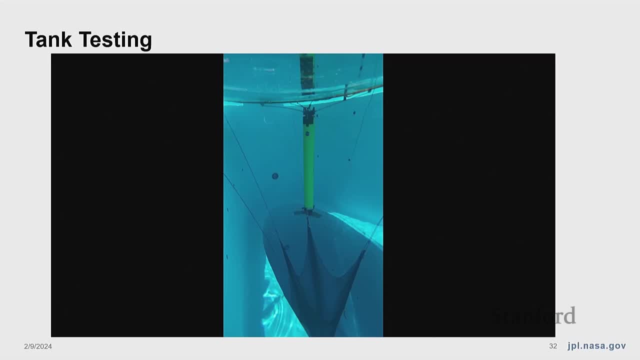 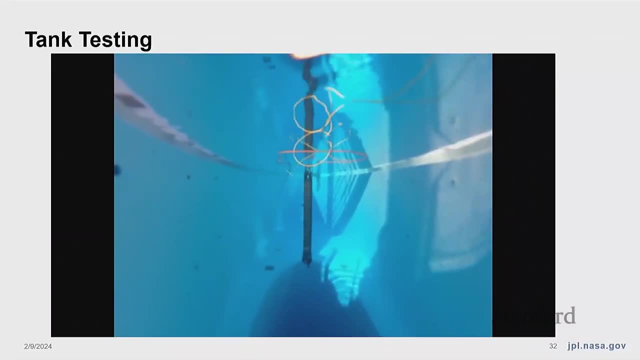 basically slowly melt up. We actually basically included the legs in the part of the vehicle that we sever. We include the legs in the piece that we sever. We rely on the buoyancy of the foam to basically keep those pieces all separate and we've simultaneously 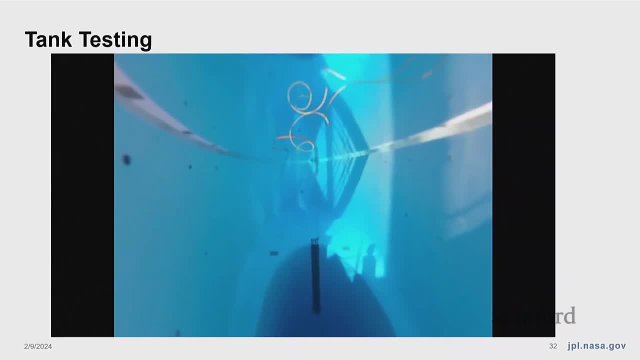 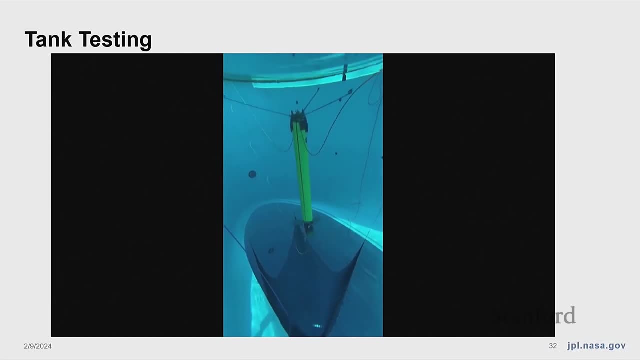 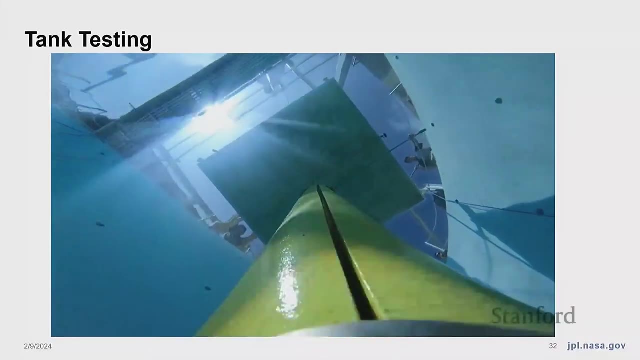 set the buoyancy engine for the vehicle to be heavy. so once we detach again- pyrotechnically detach- the top cap, you're going to see the vehicle just sink down and drift out from the bottom. This is again the landing. 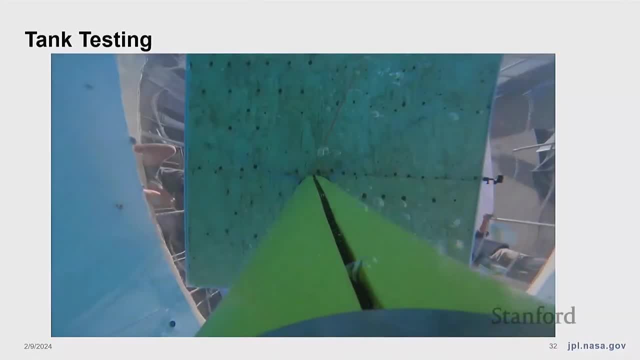 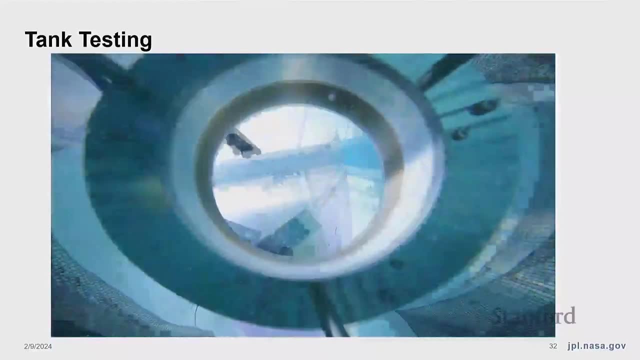 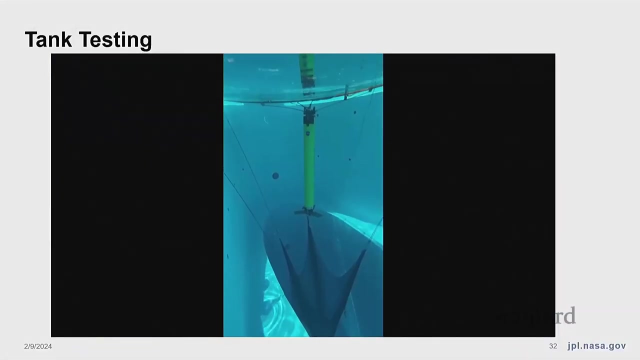 and we'll see the next slide in just a minute. So is it always the case that the surface is flat for your applications here? No, we do have basically an upward looking instrument so we can see a little bit of the ice properties. 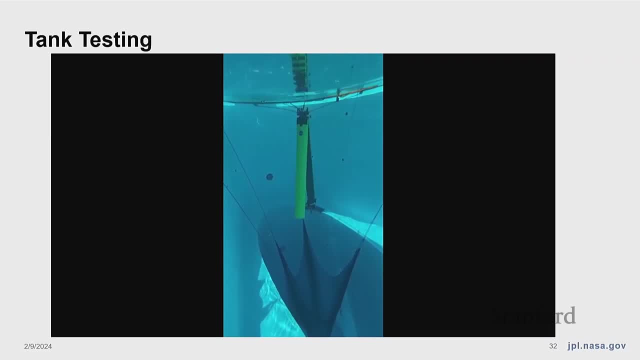 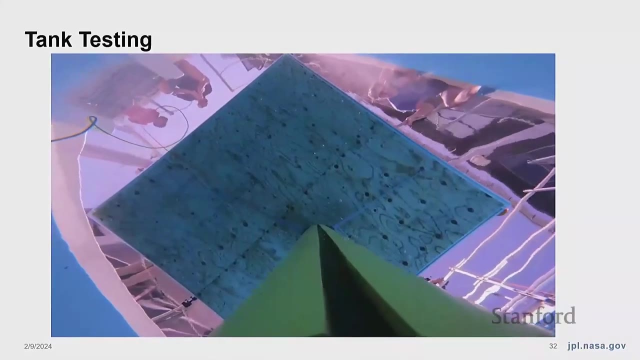 and again, those legs are each individually compliant and spring loaded so they have the ability to conform up to some level of roughness of the ice. So again, the big focus here is on simplicity. We have one real degree of freedom and then two pyrotechnically. 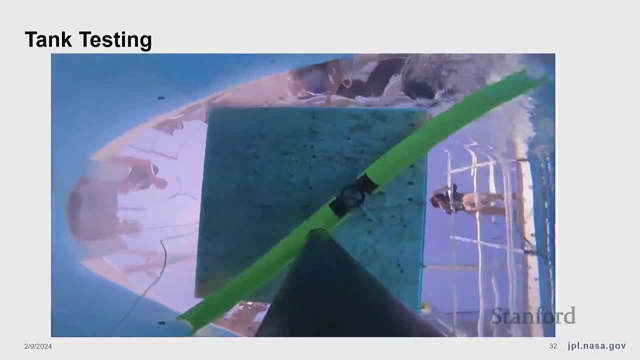 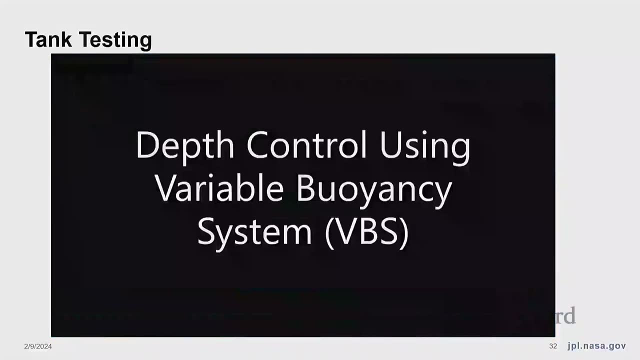 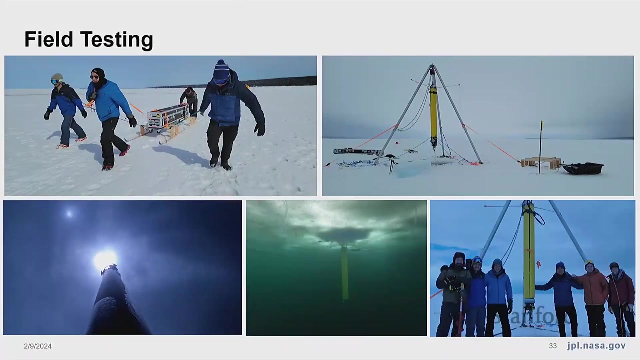 severed devices, and that's really the only control we need over the vehicle itself, Because plywood doesn't tell you a lot of scientific information. we still wanted to bring it out into the field and test there. Here we are doing a deployment up in the upper peninsula. 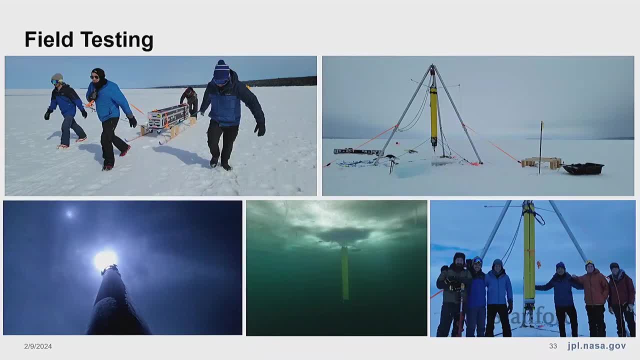 of Michigan. We drilled a borehole through ice on Lake Superior. This was frozen over and part of it was frozen over in March And we took data for a period of a couple days. There's not a lot of interesting melt data that you're going to see. 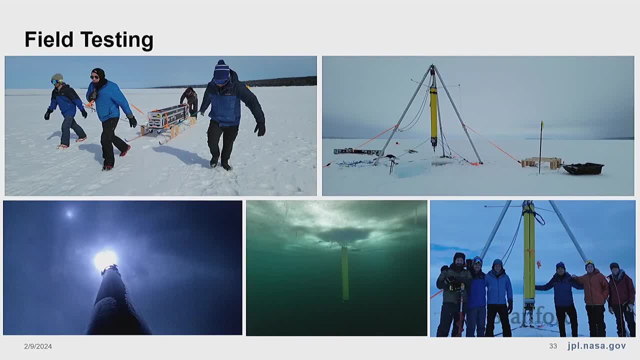 in this kind of environment. but at least let us check out both the vehicle functionality overall and how it works. So there's no real concern about catching an ice ledge with one of the legs and that flipping your instrument on its side. Yeah, so we do have upward facing instruments. 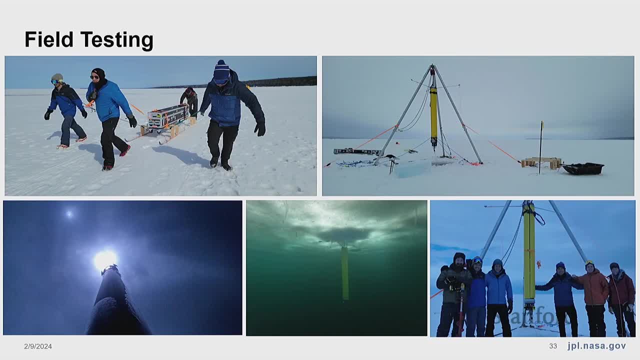 to basically try to track what that ice surface would look like. Do you have any thrusters or ways to adapt once you sense that information? It would be. don't, so we would basically rise through the VBS standoff distance of 30 meters below the ice. 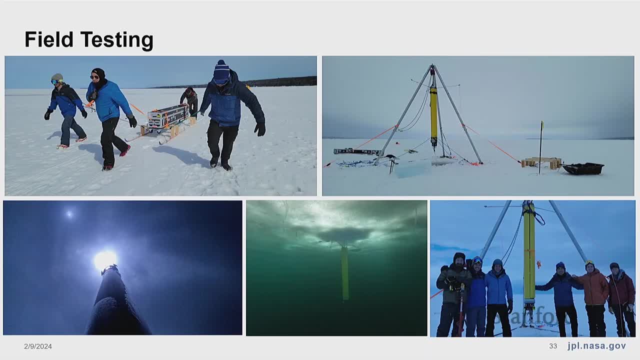 at which point, if the ice looks good, you can sever the ballast, and if not, you would keep drifting and then sever it a little bit later when you're on a friendlier landing terrain. This is actually a perfect transition, because at the end of my slides, 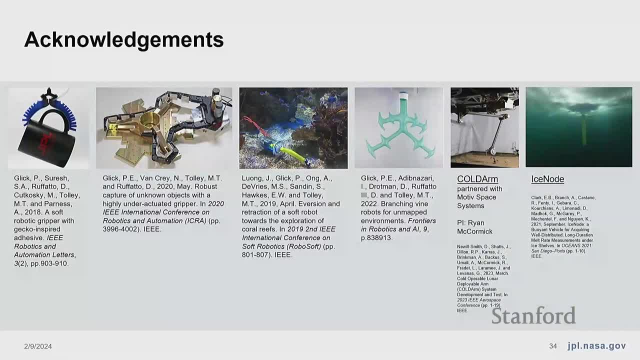 I want to thank everyone who contributed to my work from my PhD and especially my two projects at JPL had a huge number of collaborators. both of these were started before I joined, so a lot of people to thank there, as well as, of course, the research here at Stanford that I've been. 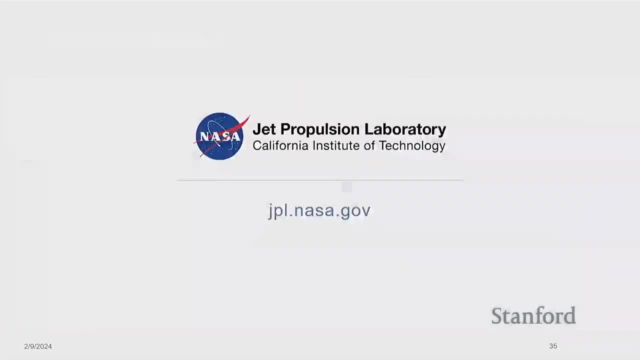 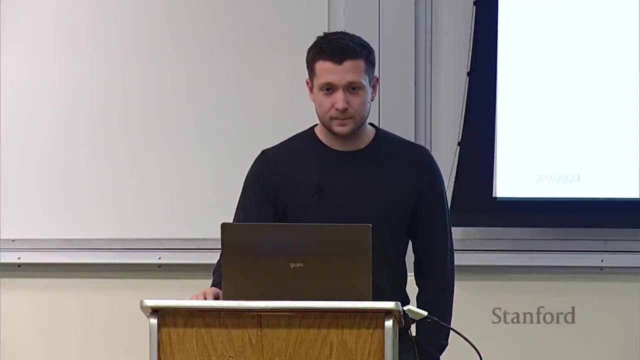 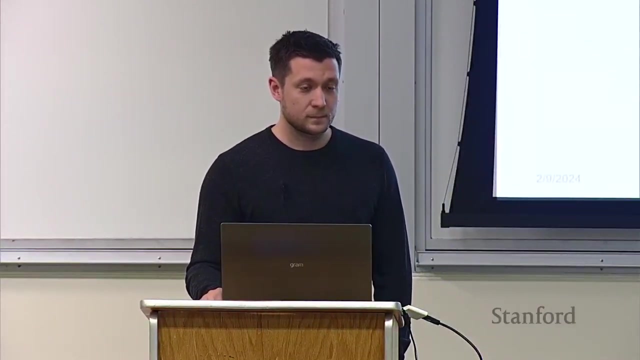 fortunate to be able to collaborate with. So thank you all for your time and attention. I'd be very happy to answer any questions. Yeah, go ahead. I'm just curious: with the branching incredible robot, did you guys try to take it to a standard rock climbing? 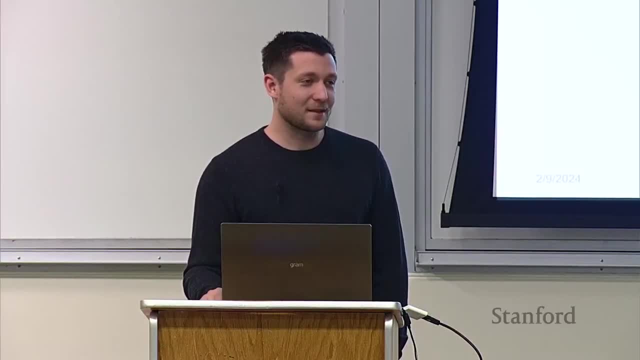 gym and see what it could do. No, I don't think that the branching would have been that helpful for rock climbing gym, because it really benefits from constrained spaces. and then the friction that you get wrapping around an obstacle, That was really so I do a little bit of. 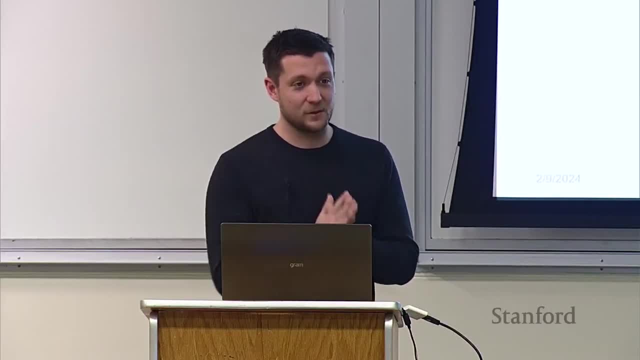 rock climbing as a hobby on the side and that was really the motivation for a stand alone pouch anchor right. so if we- yeah, basically right, in rock climbing they use a lot of cams, so carefully placed things where, basically as you put them in the